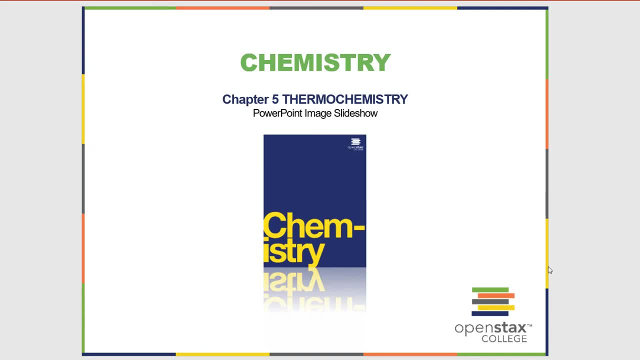 In this section we're going to look at thermochemistry. So far in this course we've looked at chemical reactions in terms of balanced chemical equations, the massive product that we could form, the concentration of some analyte in a titration, or things like this. But now we want to look at some of the energy. 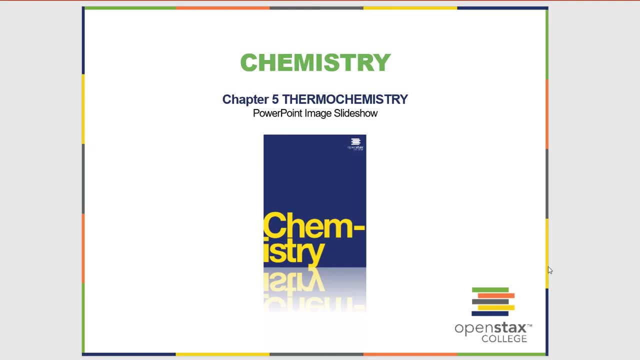 transitions that occur in chemical reactions, and this section is kind of an introduction to that to give you an idea of how scientists think about thermodynamics in general, some of the physics that applies to thermodynamics as well as later on in the chapter looking at actual enthalpy changes of 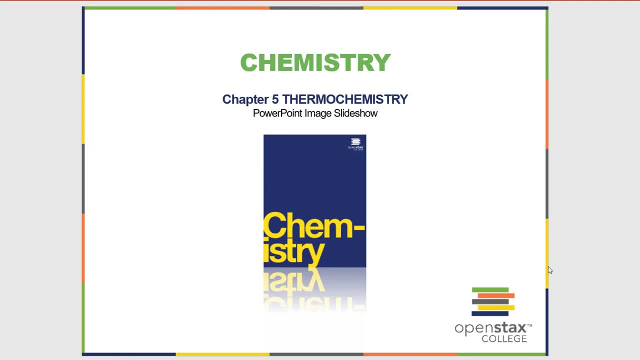 chemical reactions And thermochemistry is something you start in general chemistry 1, but you cover it in more detail as well in general chemistry 2, because there are some other factors, such as enthalpy which can be used in Gibbs, free energy, and these concepts are covered in general chemistry 2.. So this 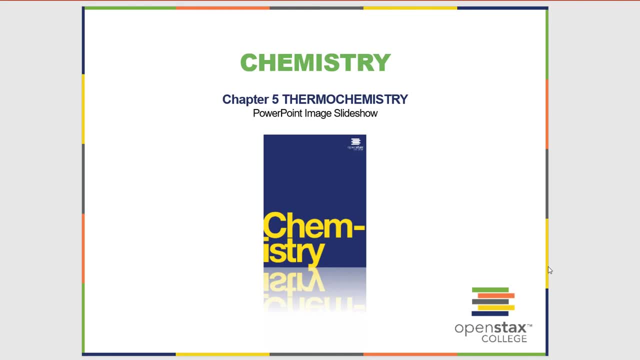 is this section? this chapter is designed to give you an introduction to thermochemistry and how chemists consider the energy change, which is another very important piece of chemical reactions. In fact, earlier in the course we talked about how you form stable products. Well, thermochemistry allows us to understand what those stable products. 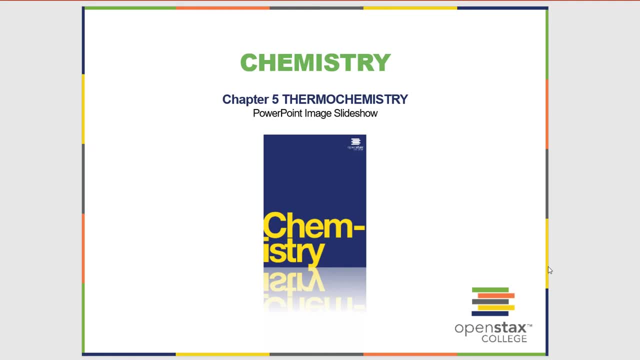 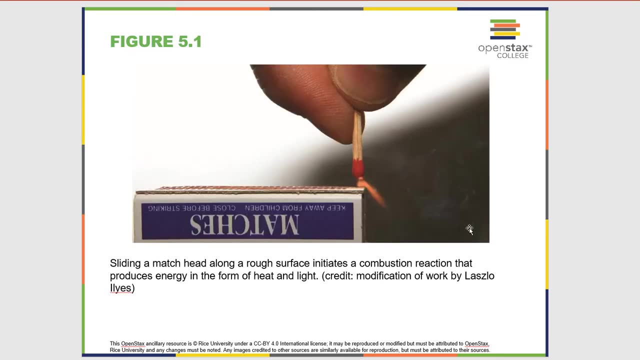 are and kind of from an energy perspective, why they're the stable products. So in this first slide we have someone lighting a match and what we have here is, inside of the match head and in the wood, chemicals with relatively high potential energy. So they. 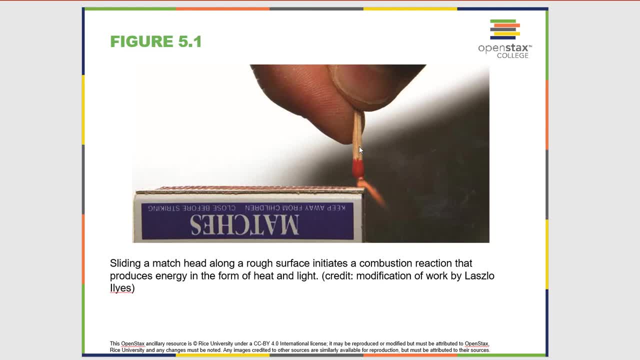 have the capacity to create heat and possibly to do work in a chemical reaction, and when the person strikes this match, these chemicals start to react and the products that form, which, if it's the burning of the wood, or mostly carbon dioxide and water, are the ones that create heat and then the 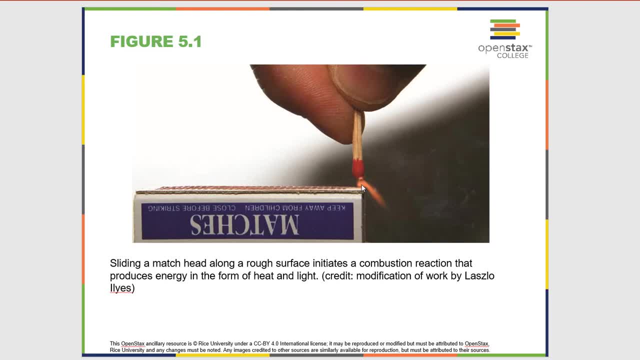 to be lower in energy than the starting materials of the wood, And there's also a chemical reactions going on in the head of the match which gives it enough energy to catch the wood on fire. So this is just one example of a chemical reaction where there's a clear and obvious energy change. Here you could see 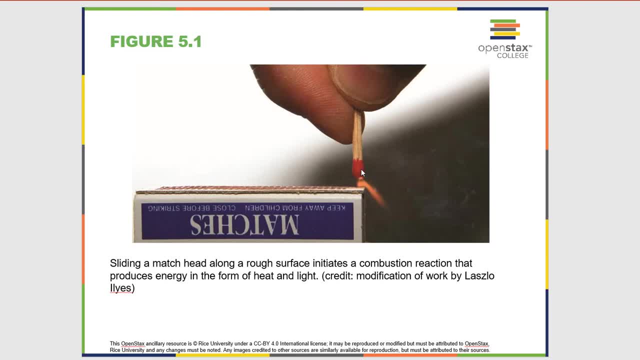 an obvious energy change, because you can feel the heat of the match and you can see the light that is being given off, So that energy has to come from somewhere, and where it comes from is rearranging chemical bonds. So in the case of here in 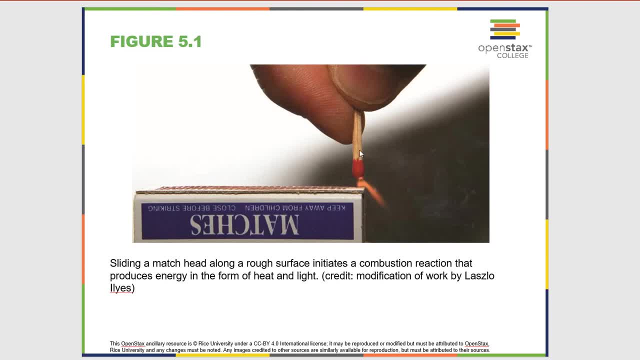 the wood of the match. you have carbons bonded to carbons When those carbons start to bond to oxygens and those carbons are also bound to hydrogens. when those hydrogens start to bond to oxygens and you form carbon dioxide and water in. 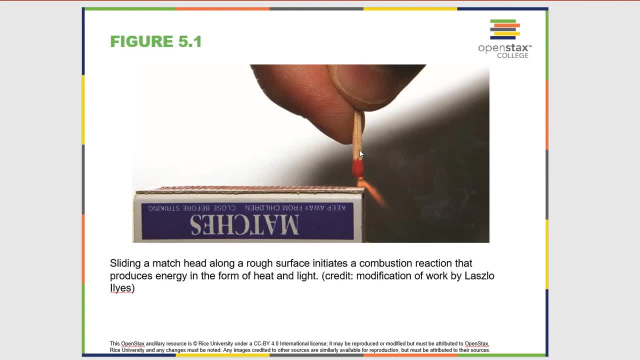 a combustion reaction. the energy of carbon dioxide and water is lower than the energy of the molecules in the wood. That energy is given off as heat and light, which you can see. Human beings take advantage of this concept all the time. This is how a car 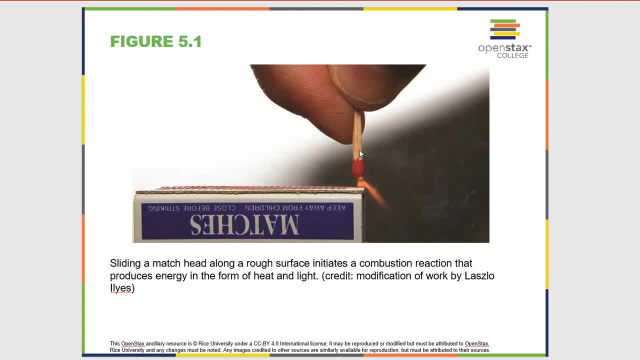 goes down the road. The energy of the gasoline is relatively high. the potential energy of the gasoline is relatively high. What's coming out of the exhaust pipe is carbon dioxide and water, which is relatively low in energy, So that energy that's given off is used to propel, something that weighs, you know. 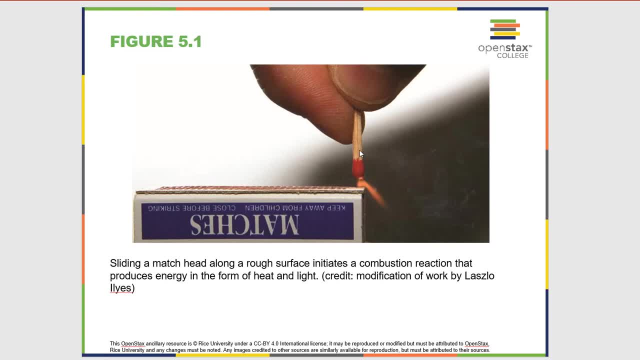 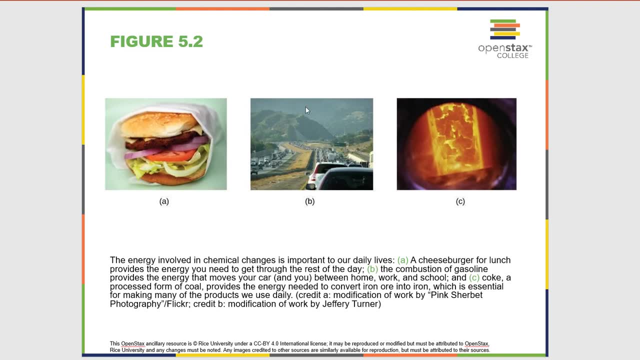 a small car 3000 pounds down the road. So that's basically how it's working. Here's are some other examples of things where energy is important. Energy is important in food. In fact, if you go to the grocery store and you look at any food product, 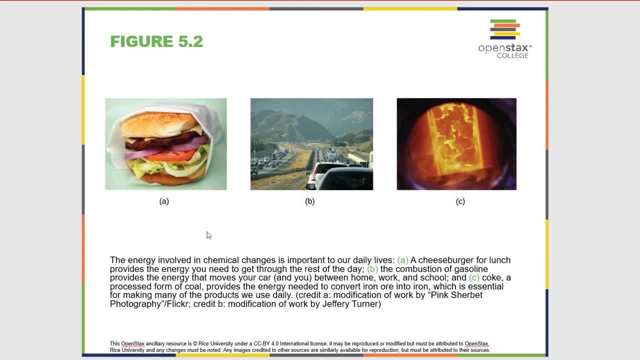 or some packaged food product, you'll see that it has energy labels right on it. how many calories that is. Believe it or not, as we'll learn a little bit later in this chapter. if you burn this food, you get the exact same amount of energy out. 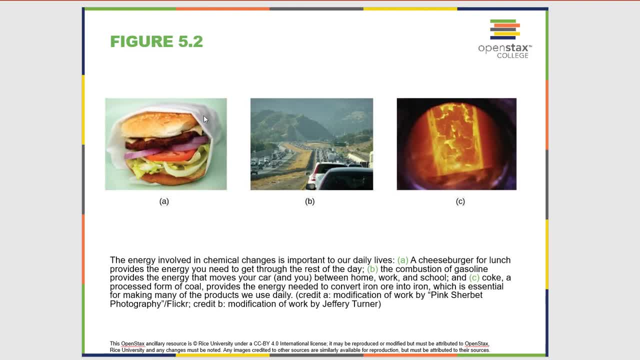 as if you eat it. So you're essentially in your body, burning it, if you will, by using enzymes. so it's a relatively low temperature burn. it's not the same as catching it on fire, but you do get the same amount of energy, And we already 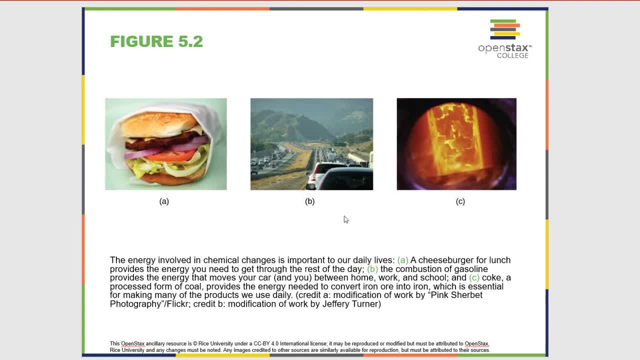 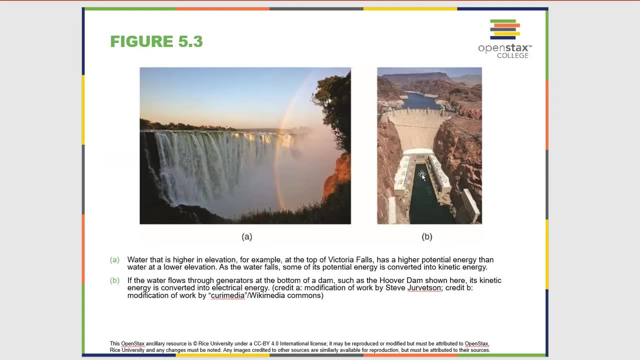 talked about. this energy is used to propel cars down the road. here someone's using heat energy to create steel, which is very important. So the energetics of chemical reactions, which were first studied now, are also extremely important to chemistry and influence a lot what is going on. Here's an example of chemical 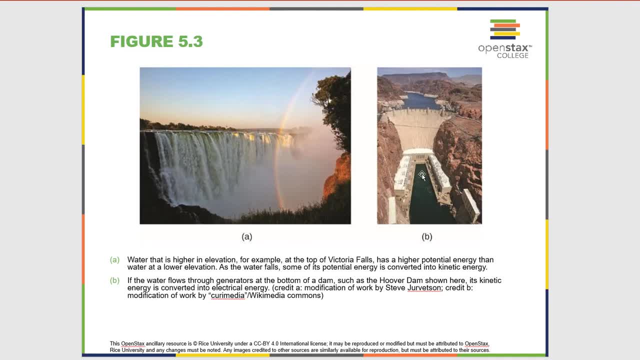 or, excuse me, general potential and kinetic energy. So potential energy is the energy of position. So in the case of the waterfall here, this water up here has relatively high gravitational potential energy. Then kinetic energy is the energy of motion. So as this water falls off the waterfall it starts to move and it gets. 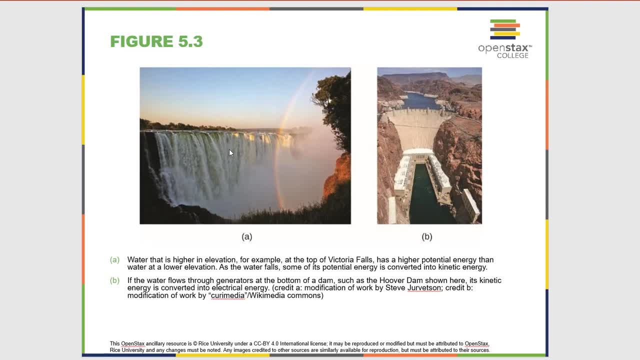 the energy of motion. It is losing its potential energy as it falls to this lower place, Because it has less gravitational potential energy, because it's less high up, It has less potential energy, but the energy it gains is this energy of motion. 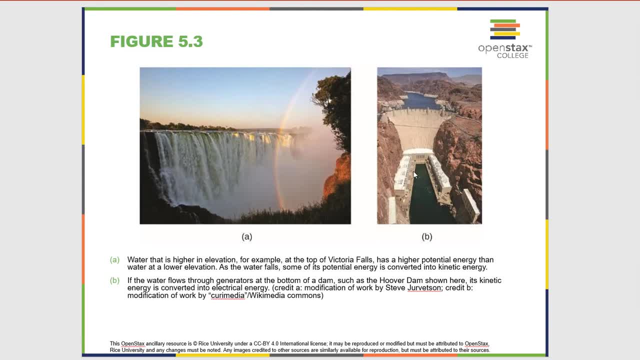 And here's a example of a dam, a Hoover Dam, which someone is taking advantage of that. We have water here at relatively high potential energy, water here, a relatively low potential energy, and using turbines which spin basically wires around magnets, you can create electrical energy. So if you're using a 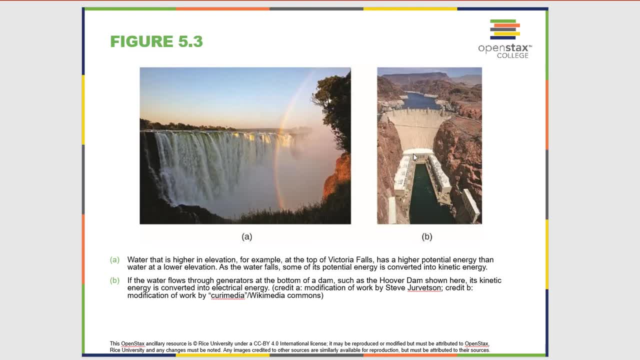 and the Hoover Dam creates quite a lot of electricity, and that energy comes from the potential energy of high water- relatively high gravitational potential energy, and low water- relatively low gravitational potential energy. Now, chemists don't really think about potential energy in terms of the energy. 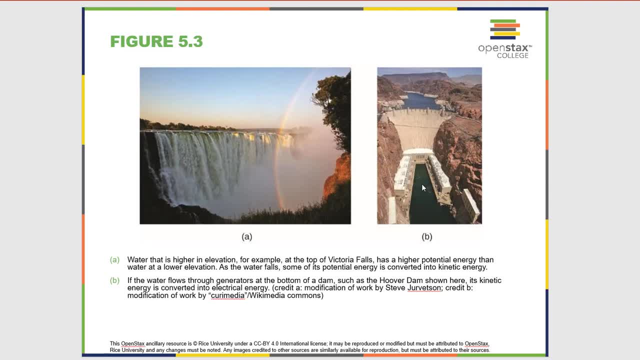 of position in terms of gravity. What they think about it is in terms of the energy of position in terms of chemical bonds. So if you have a carbon bonded to a hydrogen or a carbon bonded to a carbon, that's relatively high potential energy. A carbon bonded to an oxygen is relatively low potential. 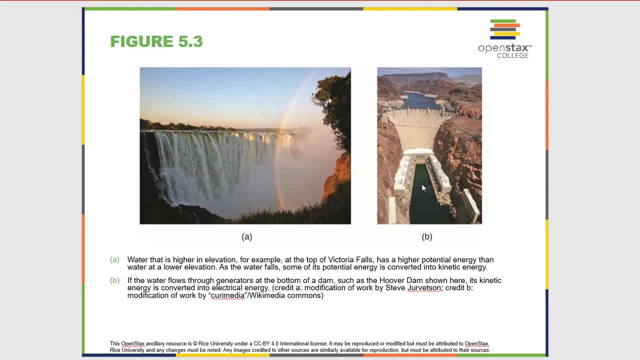 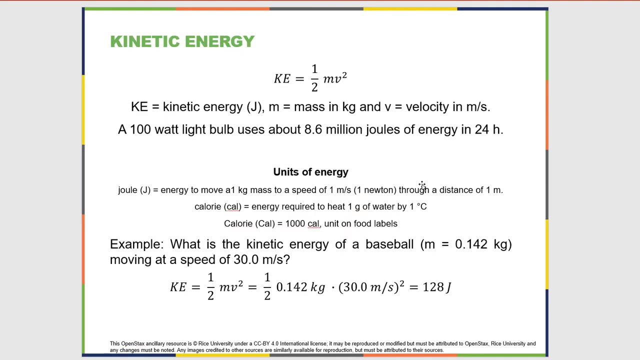 energy. So in a combustion reaction where you can change from carbons bonded to carbons and carbons bonded to hydrogens to carbons bonded to oxygens and hydrogens bonded to oxygens, that potential energy could be used to heat houses, move cars and all this kind of stuff. So one thing we do need to briefly. 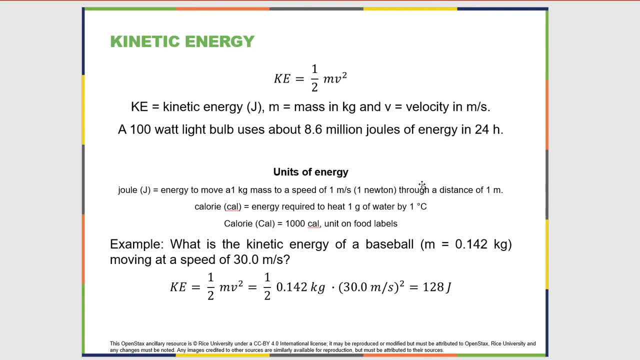 talk about. this is a physics equation, that, but it's kind of useful in chemistry, as we'll explain in a few minutes. when we talk about the thermal energy or temperature, we basically want to look at kinetic energy. So kinetic energy is the energy of motion and it has a unit of a joule, It equals one. 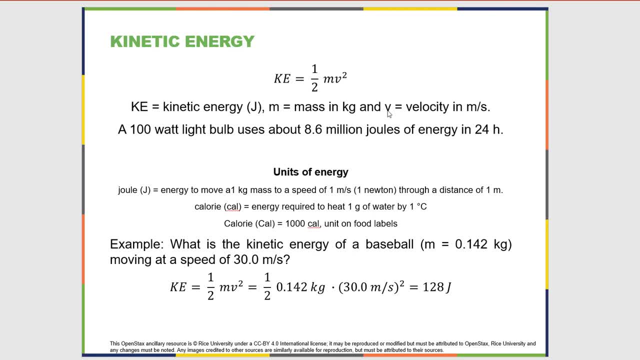 half m v squared, where m is the mass in kilograms and v is the velocity in meters per second. Just to give you some perspective. a hundred watt light bulb- okay, an old incandescent light bulb, that's 100 watts. I know new LED bulbs or 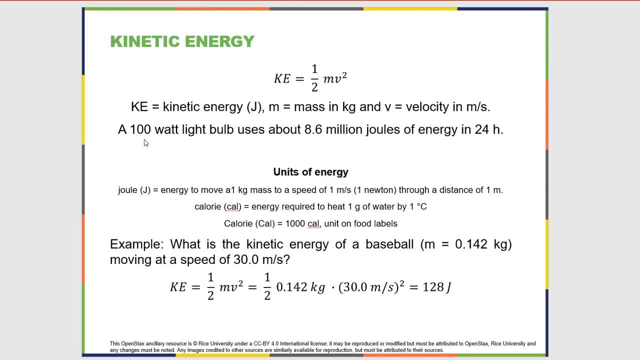 CFL bulbs are not using this much energy, but an old incandescent bulb using 100 watts uses about 8.6 million joules of energy in 24 hours. So a joule is a relatively small amount of energy And there are several units of energy, some. 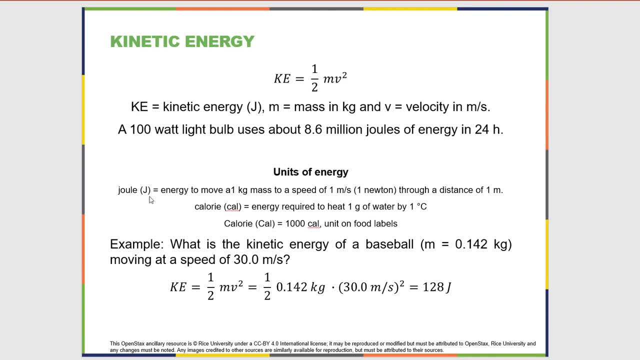 of which you're probably more familiar with, like calorie. So joule is basically energy of mass in kilograms. So you can measure energy by this and you can take the Zeal, Just because Zeal is nah, so you can measure it. the energy to move a 1 kilogram mass to a speed of 1 meters per second, that's a. 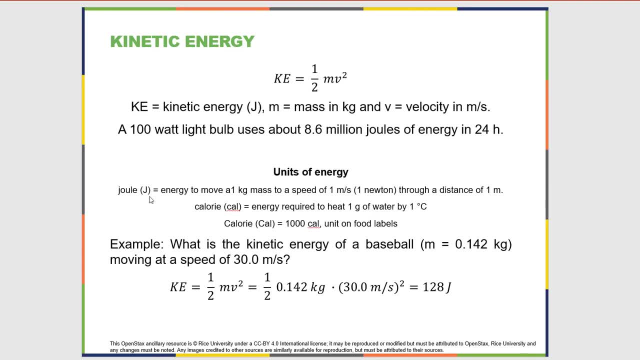 Newton the amount of energy required to accelerate a 1 kilogram mass to a speed of 1 meter per second through a distance of 1 meter. So this is the definition of a joule, Not super important, but if you do calculate this, it is 1 half mv squared. 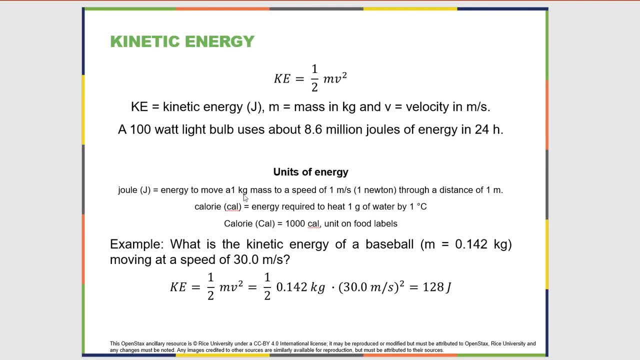 where the mass has to be in kilograms. mass has to be in kilograms and the velocity is meters per second. A calorie is the energy required to heat 1 gram of water by 1 degrees Celsius, so that's a little bit different of a unit And it's 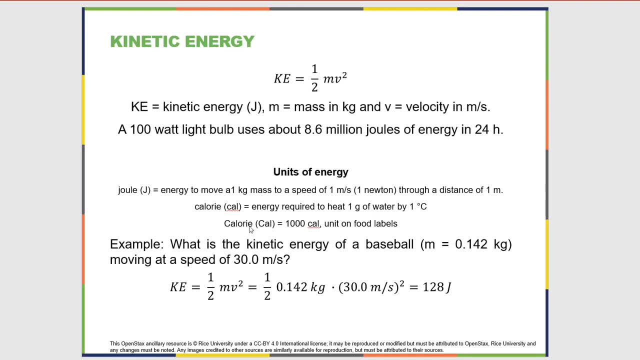 important to note that a calorie, like you see on a food nutrition label, is a thousand calories or a kilocalorie, and this is the unit used on food labels, or, said another way, it's the amount of water or amount of energy. 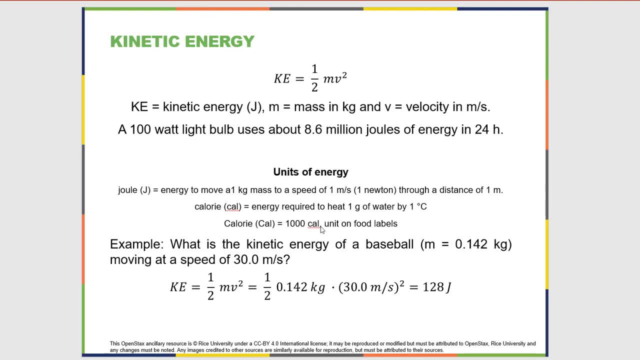 required to heat the food: 1 kilogram of water, not 1 gram of water by 1 degree C, so this is a calorie. To put this into perspective, 1 calorie is 4.18 joules, so that's. 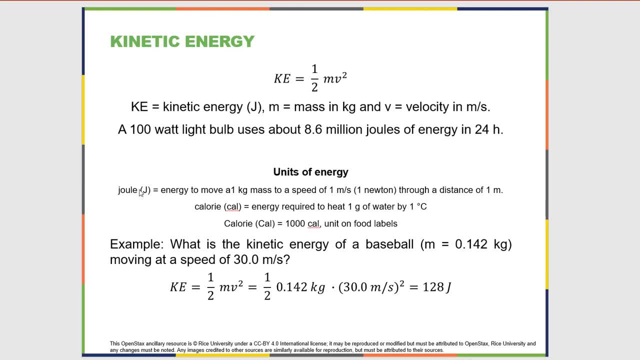 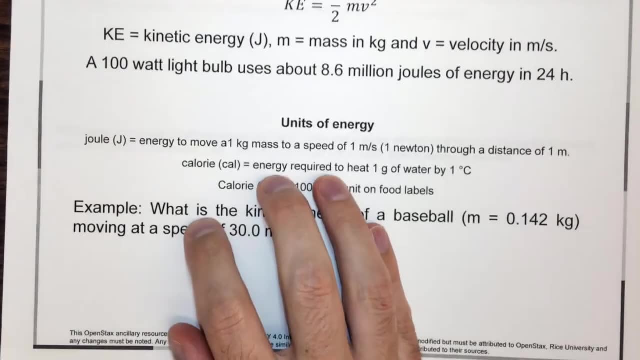 basically the relationships between this calorie and this joules. Okay, so one of these is 4.18 of these. So that gives you a little bit of perspective of some of the units of energy. Here we could calculate the kinetic energy of a baseball, and I have the same slide. I just printed it out so I could write on. 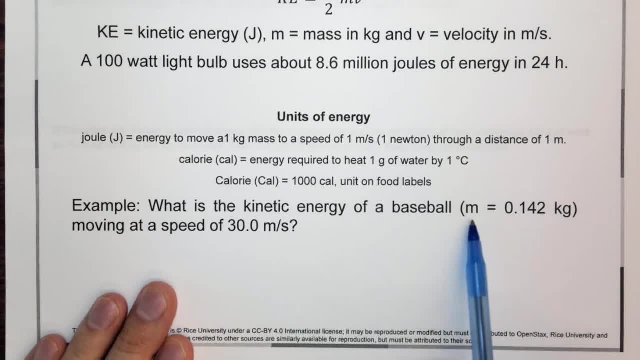 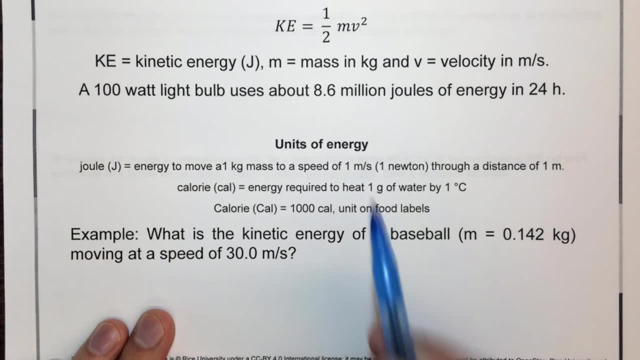 it. it says: what is the kinetic energy of a baseball? mass equals zero point one for two kilograms moving at a speed of 30 meters per second. Well, we want to use this equation: kinetic energy equals one half mass times velocity squared, And we 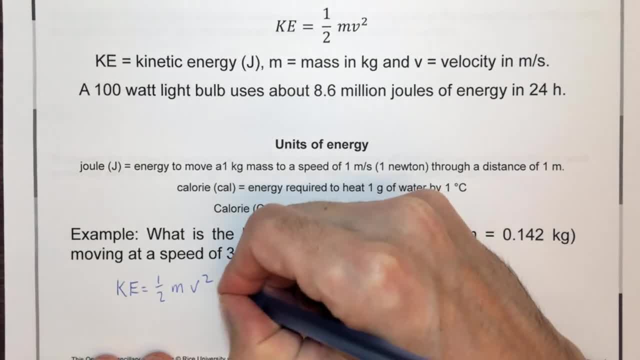 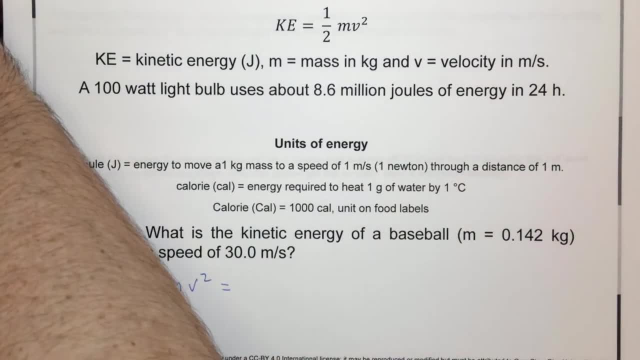 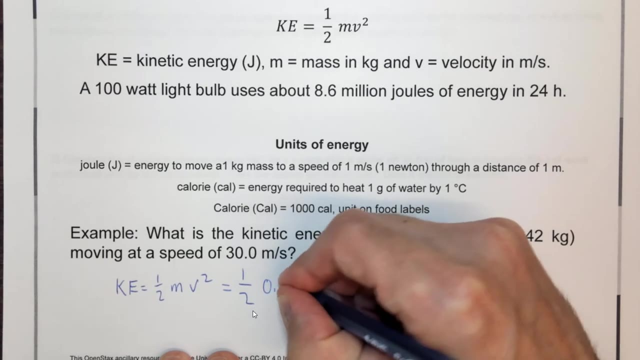 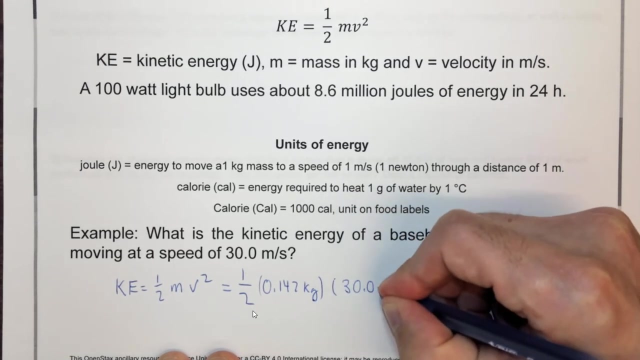 just want to simply plug in these numbers. So it's equal to however many, equal to one half the mass, 0.142 kilograms times the velocity squared, which is 30 meters per second squared. 30 squared is 900 times 0.142. times a half equals 63.9. 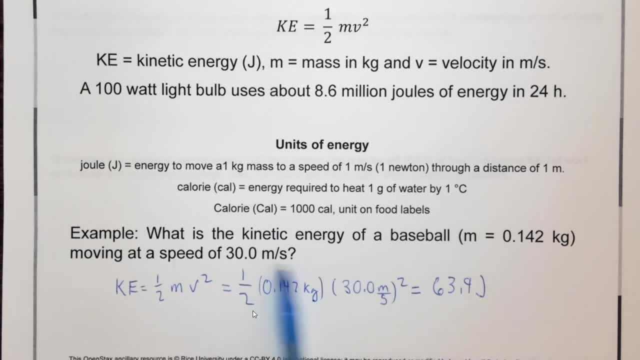 joules. So this is the kinetic energy of a baseball moving at 60 meters, 30 meters per second, which is give or take 60 miles an hour. So it's not real, real fast for a professional pitcher, but it is not slow either. but a baseball is relatively. 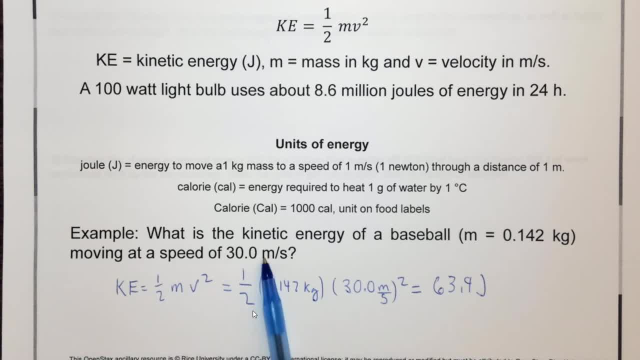 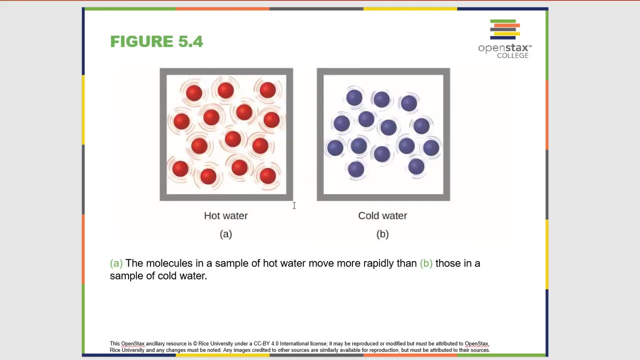 light. You can imagine if you use the car moving at 30 meters per second, the kinetic energy would be much greater because a car is much more massive than a baseball. So this just gives you a little bit of perspective of kinetic energy. Well, how do chemists think about kinetic energy? And we think 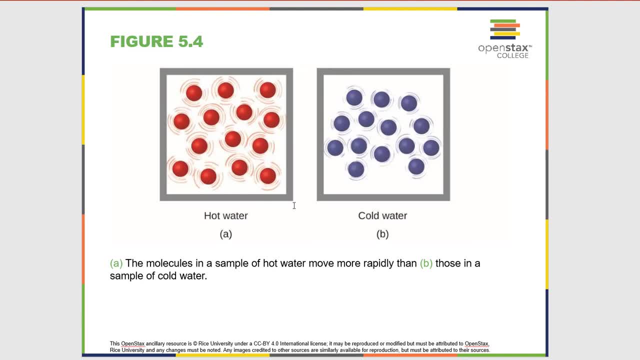 about it often in terms of temperature. So, even though you can't see it, the anything solid in front of you- you have a table or whatever in front of you- the molecules in that thing are moving And the hotter that it is, the 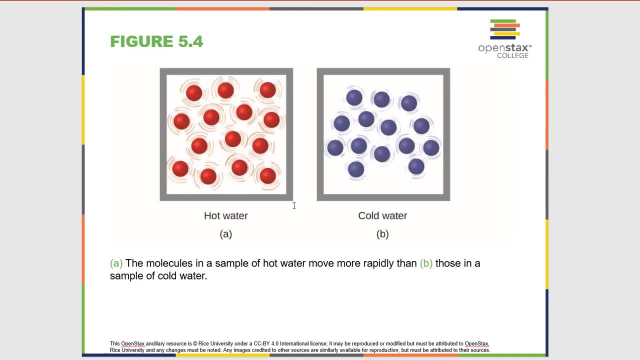 faster those molecules are moving. Remember that kinetic energy is the energy of motion And temperature is a measure of average kinetic energy. So if you have a heavy metal mass, the amount of energy that I have on the neighbors is порized and that's OK At any given temperature. there's a range of 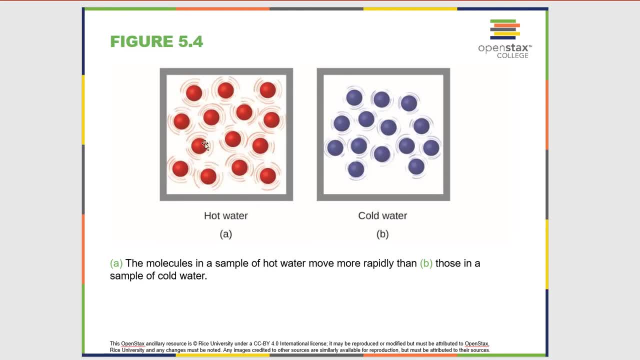 speeds of molecules. some are moving faster, some are moving slow. Now it's important to note: at any given temperature there's a range of speeds of molecules. Some are moving fast, some are moving slow, and there's an average, And that average is related to the temperature. So if you have hot water, on average, the molecules are moving faster. If you have cold water, on average, the molecules are moving slower. 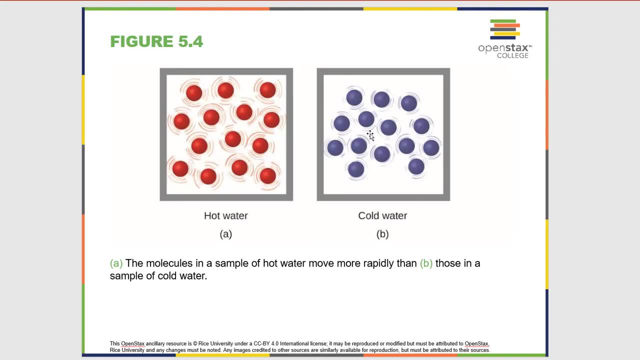 mean they're not moving. In fact, at any temperature above absolute zero- absolute zero is the temperature at which molecular motion stops- molecules are moving, Just like if you take a piece of metal and you heat it up to a temperature less than when it starts to turn red, or something like this. you 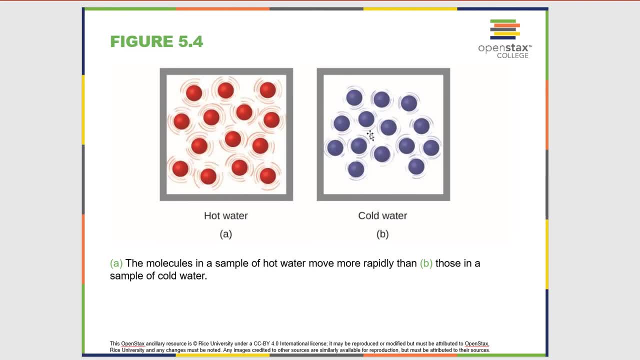 can't see that it's any hotter. So that's an important safety consideration, right? If you put a pan on a stove and you heat it up and you turn the stove off, that pan will remain hot for quite some time, even though you can't see it. So just, 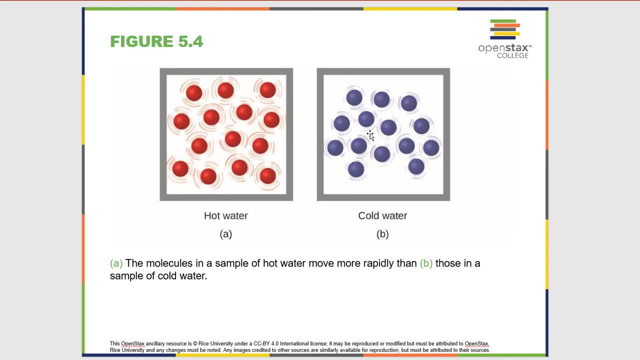 because you can't see the molecules moving doesn't mean they're not moving. Now, if you were to touch a hot pan, well, what will happen? It will burn you, And the reason that it burns you is the molecules in your hand are in nice. 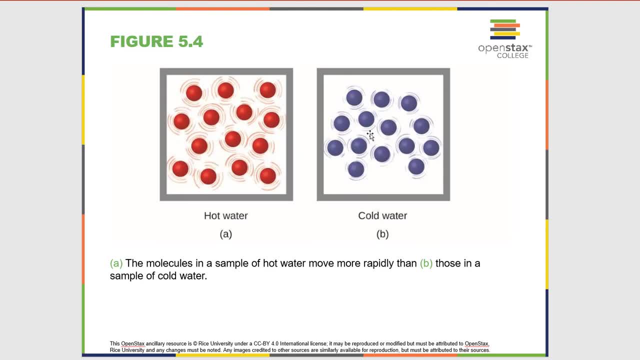 perfect alignment. If you touch something hot, they start to accelerate the molecules in your hand such that they get knocked out of that perfect alignment and we call that a burn. And what your body has to do is produce new cells that are in perfect alignment to replace those that were damaged. So 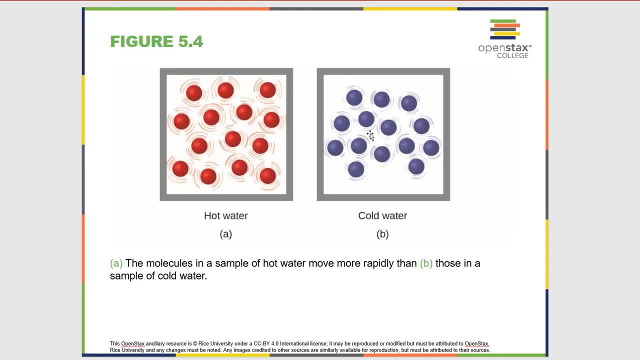 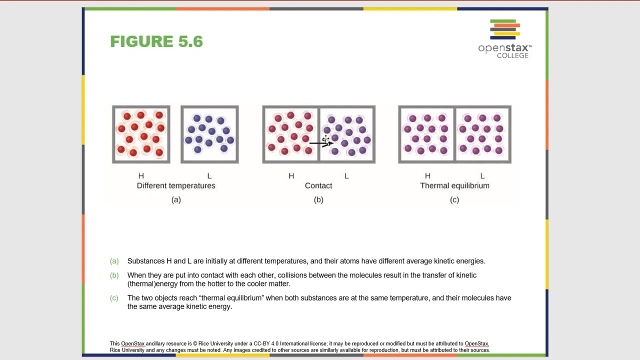 that's basically what happens, And this leads us to another important concept, which is that hot molecules and cold molecules can transfer energy to one another. In fact, usually we think of energy flow from hot to cold. So if we take a hot water and cold water and we put them in contact, we mix them together. 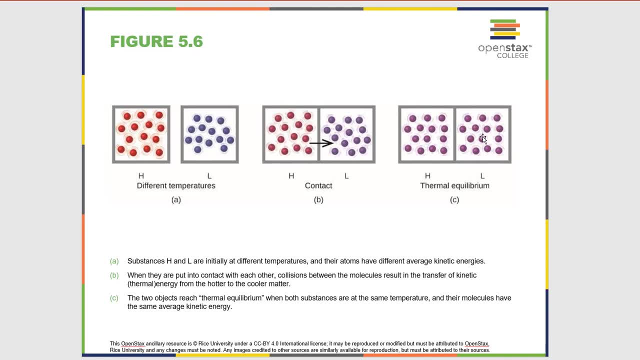 we'll reach some kind of thermal equilibrium where they're all moving at the same average speed. Now again, that doesn't mean every molecule is moving at the same speed, where every molecule has exactly the same you know amount of kinetic energy. what it means is that, on average, the average of the old, hot and 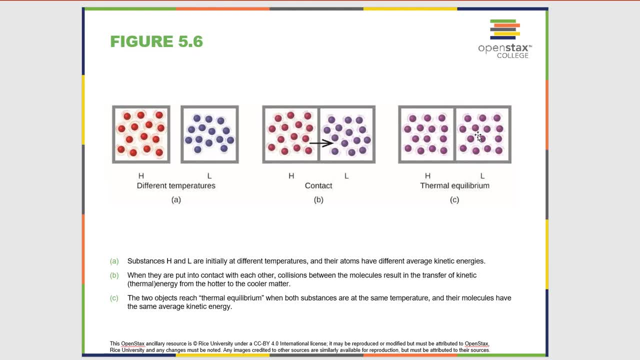 the average of the old cold will be equal, So therefore their temperatures will equilibrate. So if this is at 100 and this is at 20 and you have the same amount of each and there's no thermal loss, they'll equilibrate somewhere. 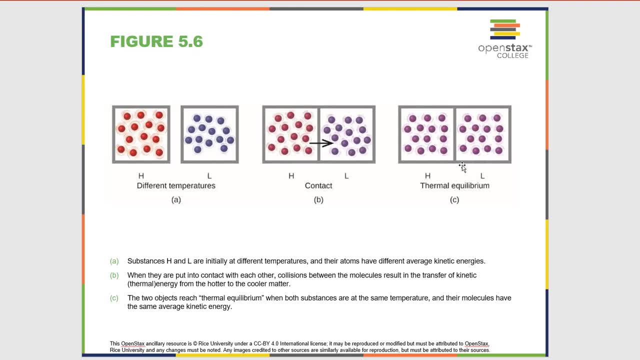 between 100 and 20.. So that's basically what happens. So this is why, if you take a hot cup of coffee and you forget to drink it in the morning or whatever, you leave it on your counter and when you come home it's not still hot, because 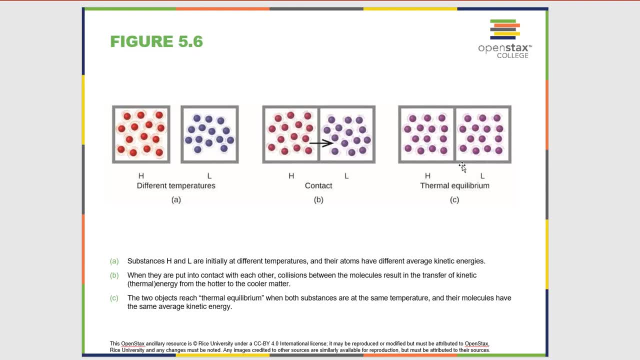 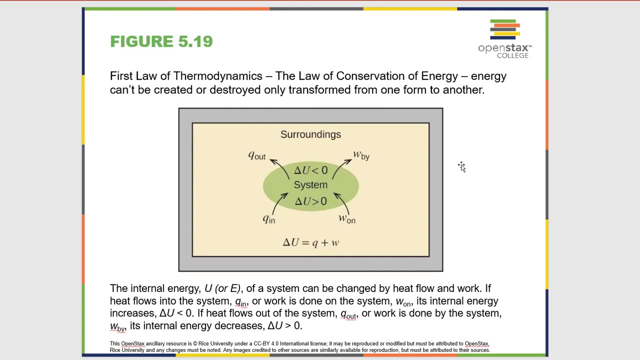 it's in contact with the surroundings, So it will slightly elevate the temperature of the surroundings- but there's a lot of surroundings, so that's not even noticeable- but it will also decrease its own temperature. So, when it comes to thermodynamics, which is the next thing that we're 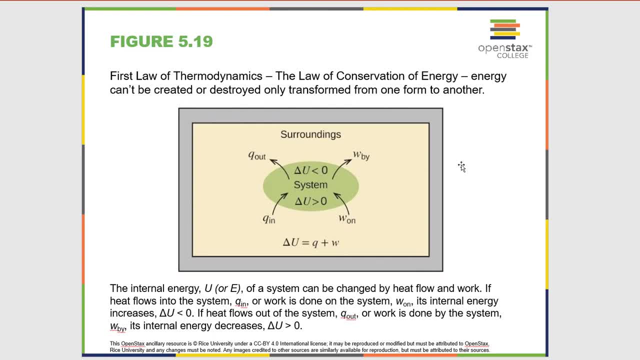 going to talk about. what we need to consider is this pesky problem of the law of conservation of energy. So the first law of thermodynamics is called the law of conservation of energy, and it says energy can't be created or destroyed, only transformed from one form to another. So when we want to study energy, 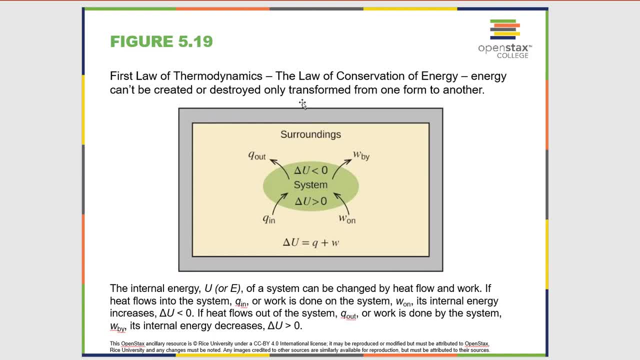 changes. this causes a problem because the overall energy change for the universe is always zero, because energy can't be created or destroyed, only change from one form to another. And we're not gonna ignore e equals mc-squared. we're in a nuclear reaction. energy mass is transformed into energy, But for 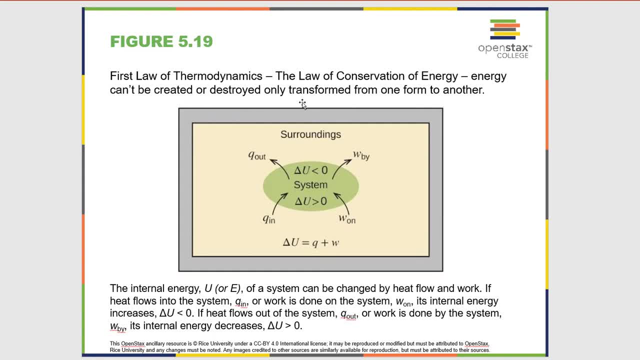 everyday type of chemical reactions, we have this problem. We don't want to have the change in energy for all reactions to be zero. That doesn't make any sense because we're doing a reaction inside of a combustion engine that's making our car go down the road. So the change in energy is important for converting from. 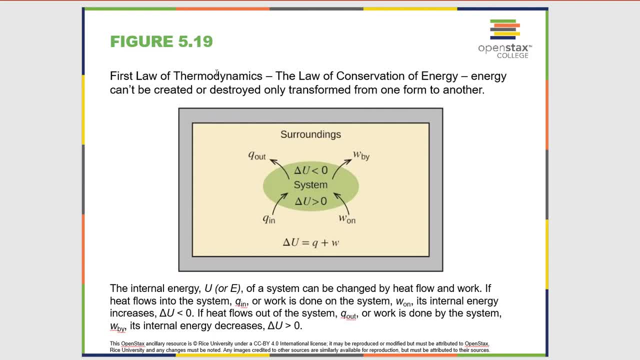 the hydrocarbon and gas to carbon dioxide and water and using that energy to propel the car down the road, And it forces us to very carefully define things. So what we have to define is the system here, the green oval and the surroundings, So we can look at the change in energy of the system and the 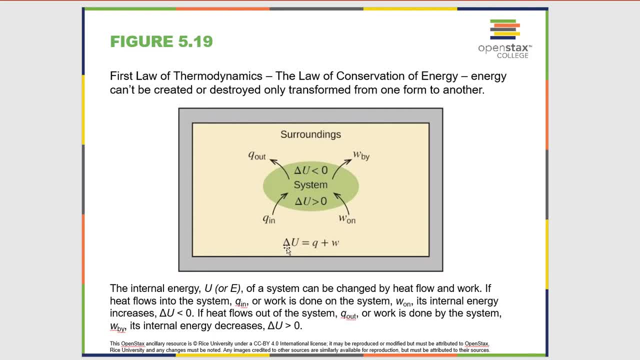 surroundings. And here we have the formula: delta U or delta E equals Q plus W, where U or E are change in internal energy, Q is heat and W is work. So this is basically what we're doing, So we're defining the system. what's happening to? 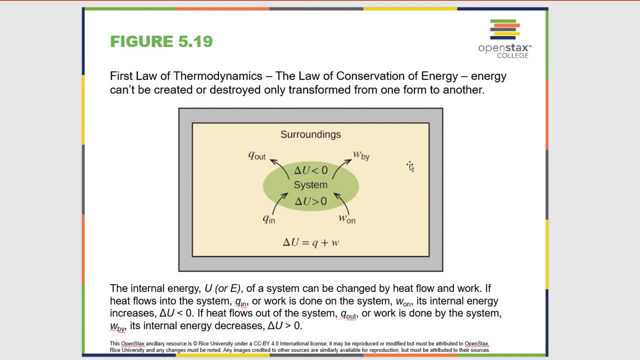 the system. and if the system loses energy, then the surroundings gain energy. And if the system gains energy, then the surroundings lose energy. So we're looking at the change in energy in terms of the system and the surroundings. In chemistry, the system is almost always a chemical reaction that is occurring, So 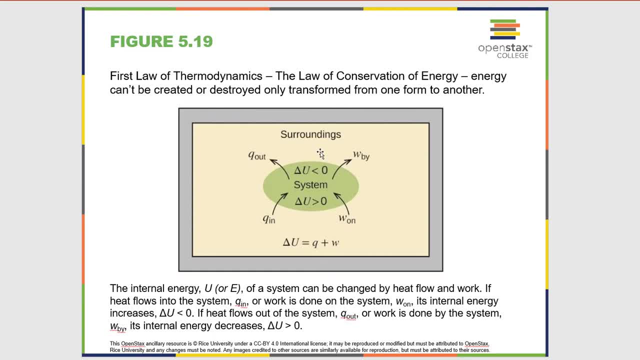 that's basically how we're going to get around this first law of thermodynamics, because the overall change in energy for the system and the surroundings is zero due to the law of conservation of energy. but the system can have a change in energy and the surroundings can have the opposite. but 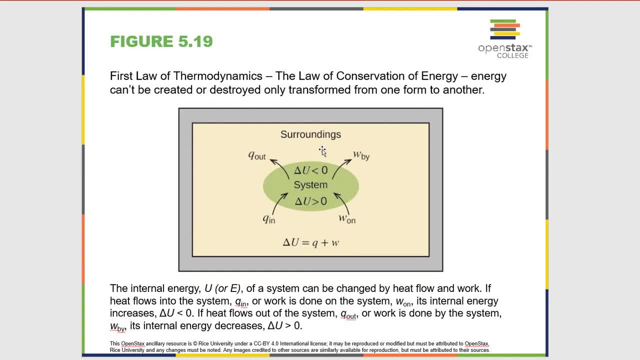 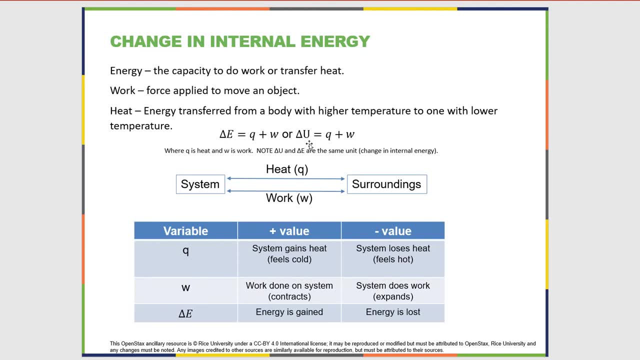 say, magnitude of change in energy, which is what chemists want to study. So let's look at this change in internal energy. I'm used to using delta E. this book uses delta U. they're the same thing. So energy is the capacity to do work or transfer heat. So energy you can think of. 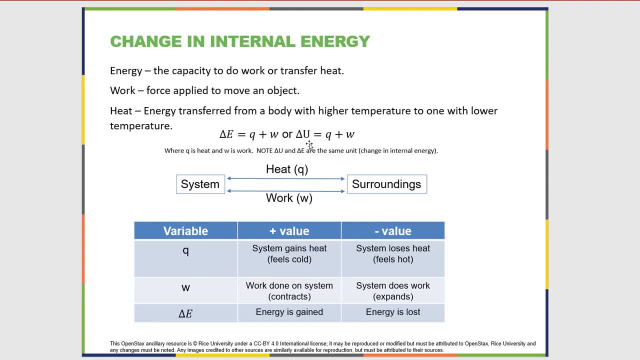 essentially as a quantity. Something can have high energy or something can have low energy. You can think of energy kind of like money- Someone could have lots of money- or because someone could have a little bit of money. Work and heat are ways to transfer money. So maybe through a check or 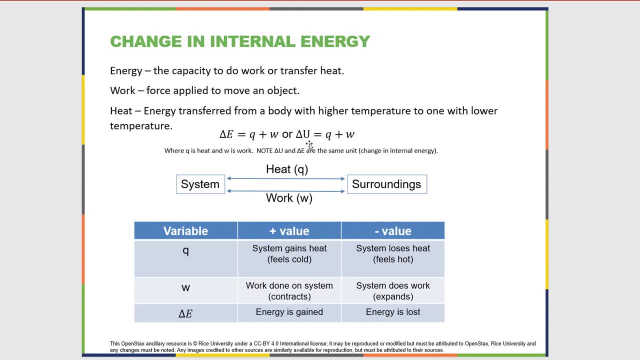 a credit card, if you will. Those are two ways that people can transfer money from one person to another. So someone with a little bit of amount of something like money could transfer or, excuse me, could have money transferred to them from someone with more money, something like this. So this is basically. energy is a. 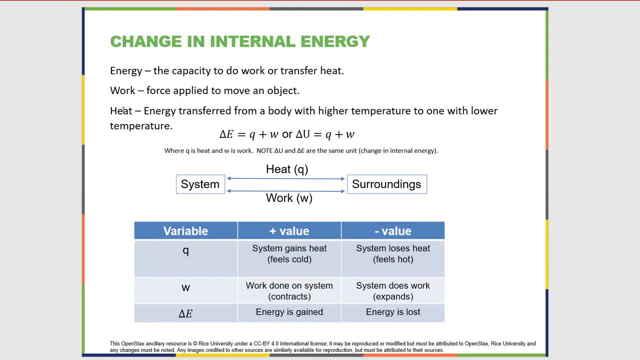 quantity, and work and heat are ways for two objects to transfer that quantity, like credit cards and cash, if you will, versus the amount of money being the quantity. So it's just kind of a general example of how this works. So what we 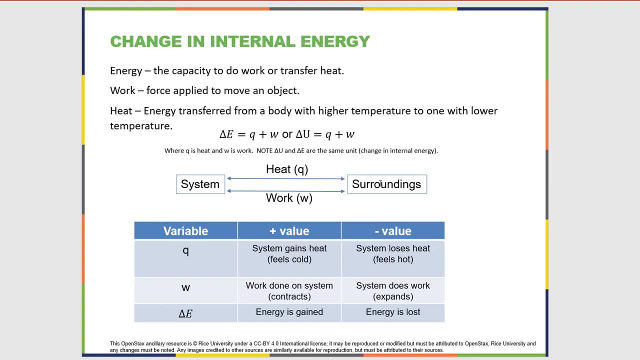 have here is we have a system and we have the surroundings And they can transfer heat between one another or they could transfer and they can transfer work between one another. So this is basically what's happening. Sometimes the system will transfer heat energy to the surroundings. sometimes the 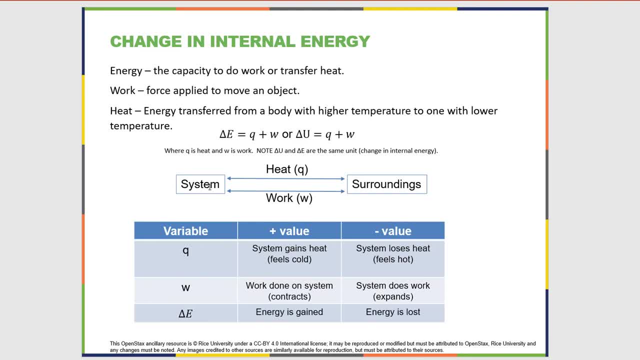 surroundings will transfer heat energy to the system and vice versa. Sometimes the system will transfer work to the surroundings and sometimes the surroundings will transfer work to the system, And it leads us to these variable definitions that we need to be familiar with, and this is super. 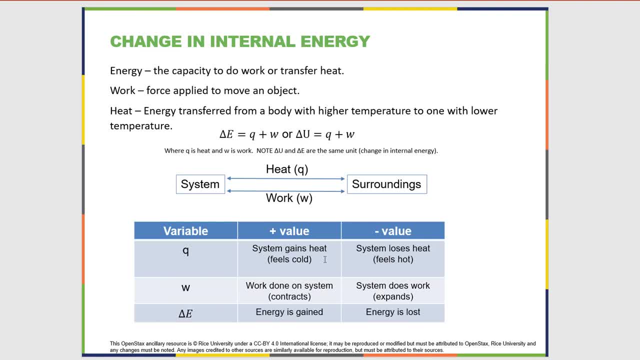 super important In terms of thermodynamic quantities. positive and negative come into play all the time and you might ask yourself: well, how can you have a negative amount of work? or how can you have a negative amount of heat? That doesn't make any sense In thermodynamics. negative doesn't actually. 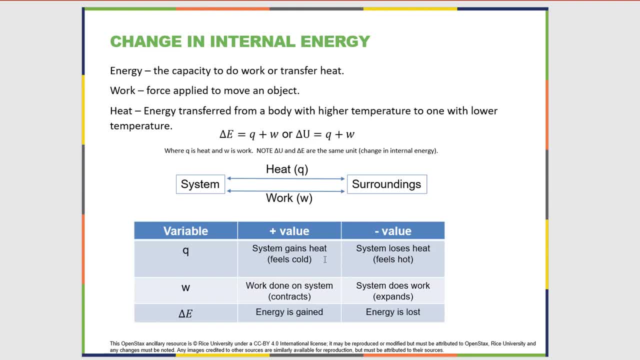 mean the quantity is negative, it means released. So if the heat or work is negative with respect to the system, it means that the system loses heat or work. If the heat or work is positive with respect to the system, it means that the 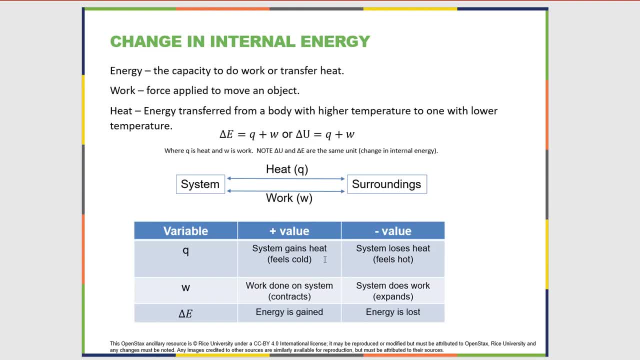 system gains heat or work. So positive or negative doesn't have anything to do with the amount, it has to do with the direction. So it's not actually negative heat, it means released heat. Note that whatever work or heat the system gains or loses, the surroundings do the opposite. So if 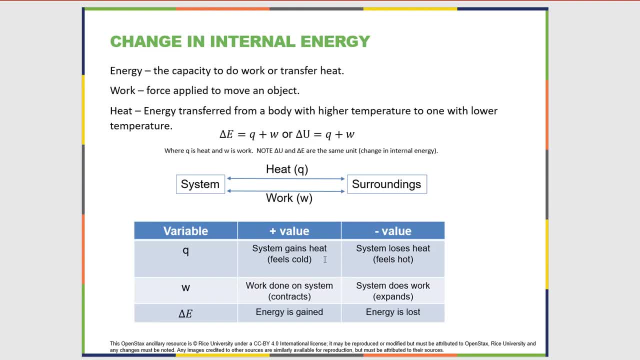 something gains a hundred. if a system gains a hundred kilojoules of heat, the surroundings must lose 100 kilojoules of heat. This creates a pesky problem when you're doing thermodynamic questions, and we'll do several examples in a. 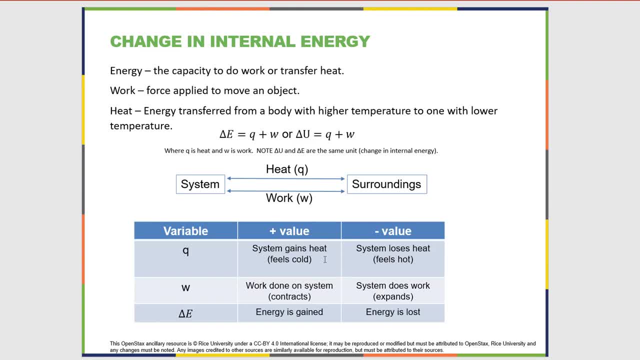 few minutes, because of the fact that we constantly need to monitor whether heat and work are positive or negative, And because it's Q plus W, which is probably the easiest equation you're ever going to learn in chemistry class. what the trick is is whether Q is positive or negative and whether W is positive or 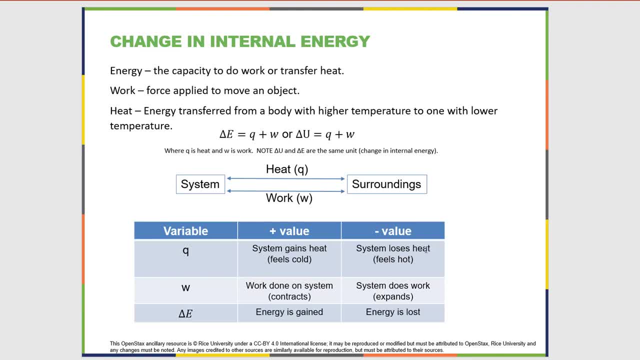 negative. So this table is designed to help us understand or remember what the values are. So if Q is positive, the system gains heat. So that's basically the system feels cold. This is counterintuitive. If something gains heat, why would it feel cold? Well, you are. 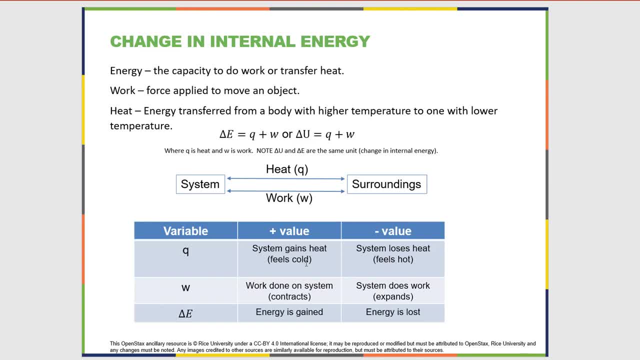 almost always the surroundings. So if you're doing a chemical reaction and you feel the vessel that it's in and it feels cold, that system is gaining heat from you, the surroundings. The reason it feels cold is it's drawing energy away. 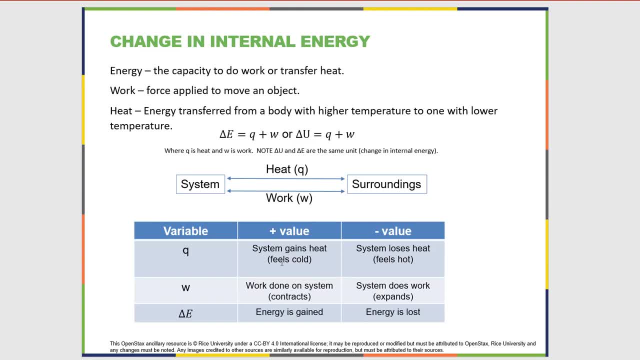 from the surroundings. So you are the surroundings. so that's why it feels cold. If this value of Q is negative, the system loses heat. the system gives off heat. Well, if you're the surroundings, you're gonna feel the heat that it's giving off and it's gonna feel hot. Work is. 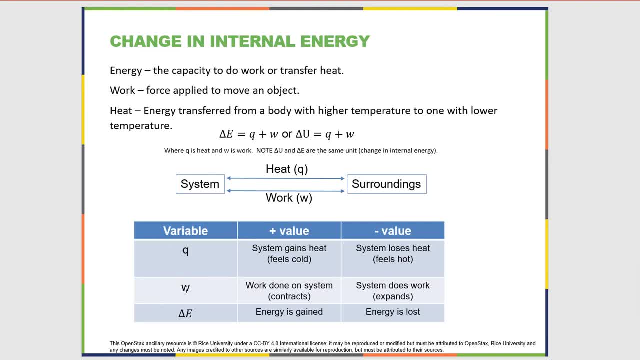 actually a force over a distance, So we need to actually have something physically move. So if work is done on a system, it contracts, it gets smaller. If the system does work, it expands, it gets bigger and theoretically the surroundings get smaller, although usually not very much relative to the 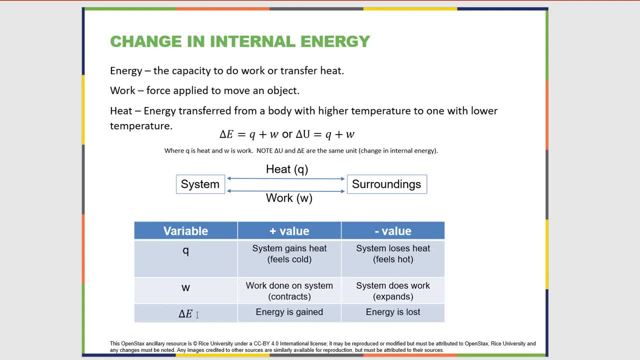 size of the surroundings, being the entire universe. Delta E- energy is gained if it's positive, and if it's negative, energy is lost. So now what we want to do is we want to look at these variables- heat and work- individually, which, remember again, heat and work are the ways to transfer energy between the 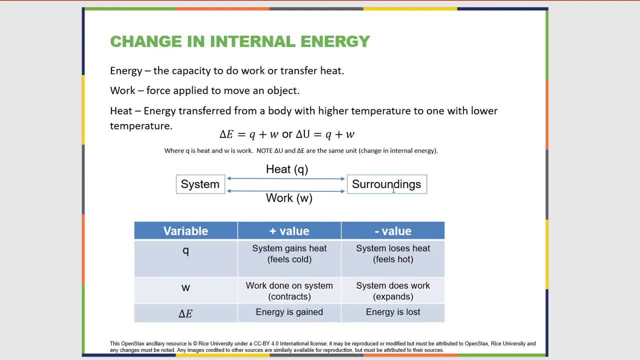 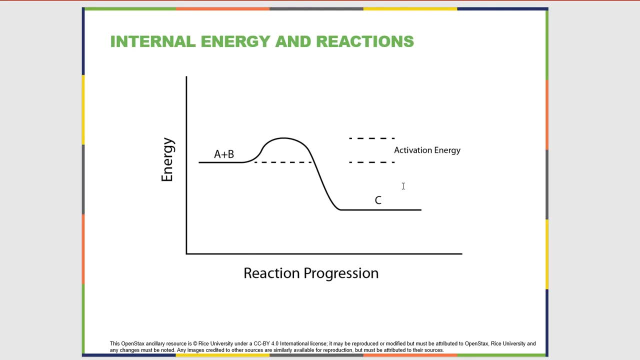 system and the surroundings, just like cash and credit cards are a way to transfer money from one person to another. Same basic idea. Now, one other thing we need to look at before we look at actually doing a few examples of these different things is we need to look at how one might view internal. 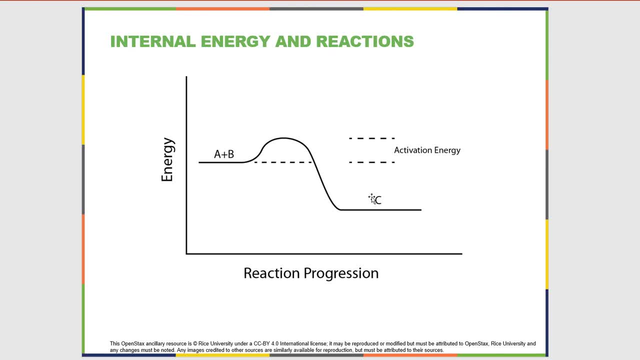 energy of a reaction. So here if we have A plus B yield C, you can see that the energy of the reaction is equal to the energy of the energy of the reaction. So here, if we have A plus B yield C, you can see here A and B are relatively high in energy and C is relatively low in 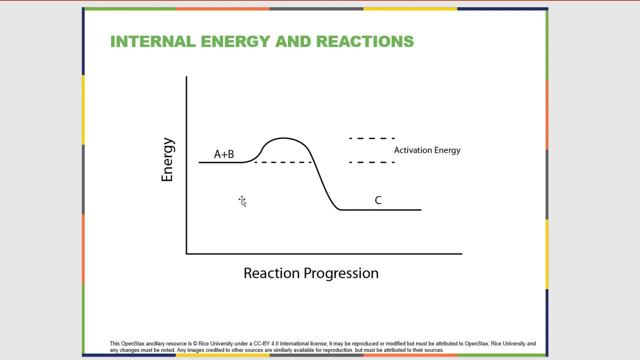 energy. So, as this reaction occurs, energy is released. If it's heat energy, this will get hot Okay. if it's Q, if it's work energy, this system will expand. So that's basically what's happening here, And this energy is released and this 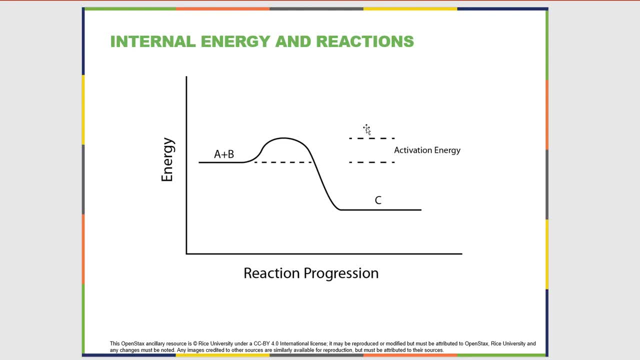 energy could be used to, for example, make a cargo go down the road. Now, if C were up here on the energy scale, notice that energy is on the y-axis. it means that you would have to put energy in to get A plus B to form C. So if you were standing near this, this would 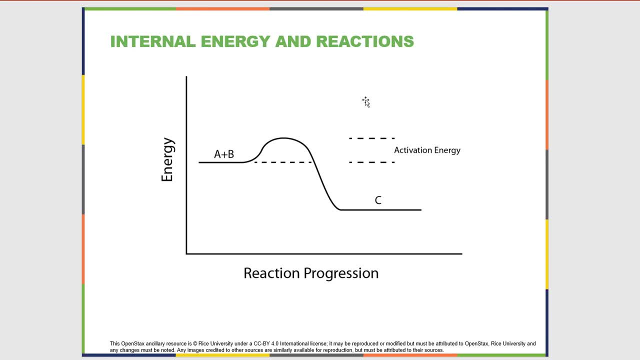 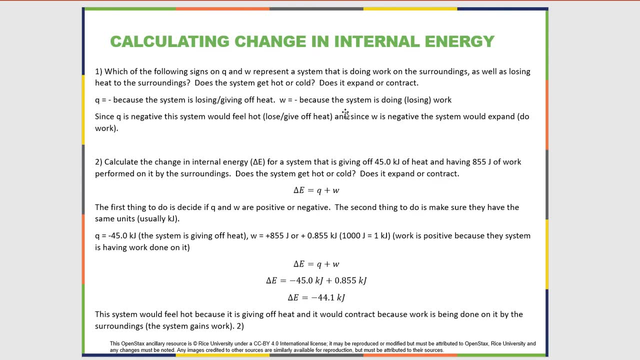 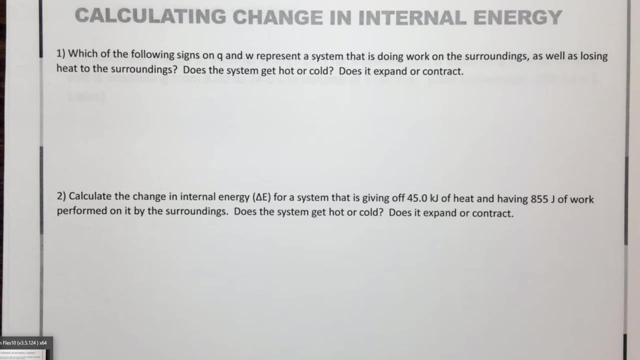 feel cold. if C was up here or if it was work energy, this system would contract because the surroundings would give it work energy. So that's basically what's happening. So now I want to look at a couple of examples where we determine the signs on these different things, and in this case, the bottom case, we actually 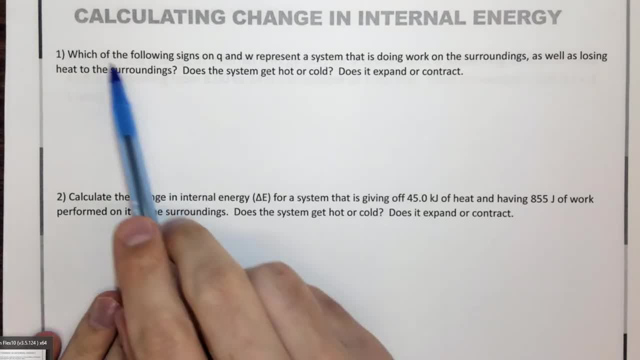 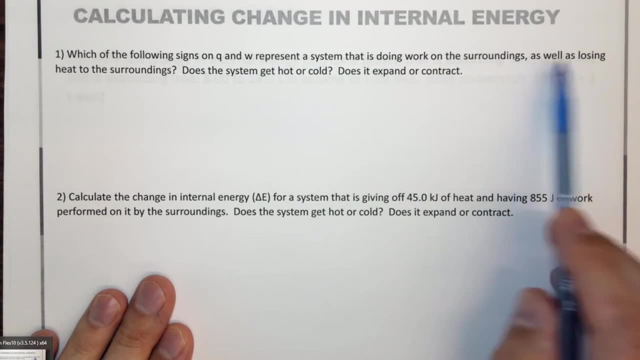 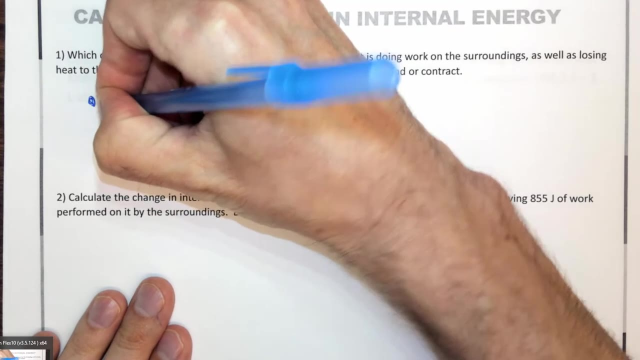 calculate change in internal energy. It says which of the following signs on Q and W represent a system that is doing work on the surroundings as well as losing heat to the surroundings. So let's look at Q and W, And for Q, which is heat. 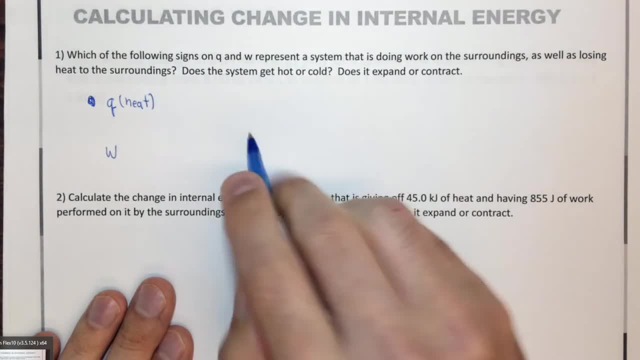 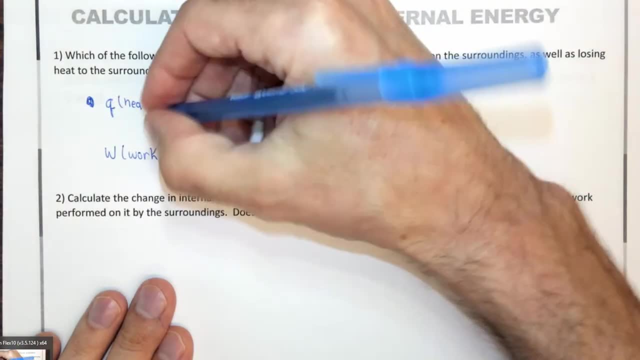 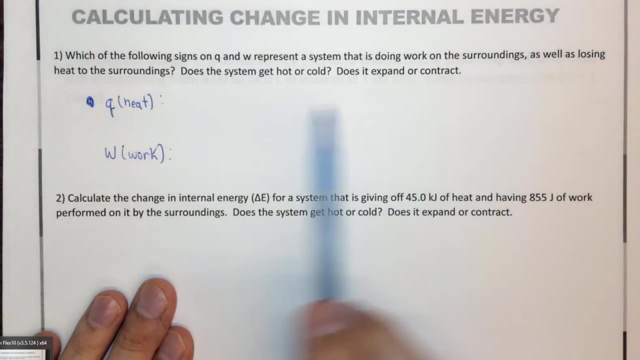 we want to also determine: does it get hot or cold? And for work W, which is work we want to see, does it expand or contract? So let's take a look here at what's going on. So for Q, we're looking at heat. So this is losing heat to the surroundings. So this is. 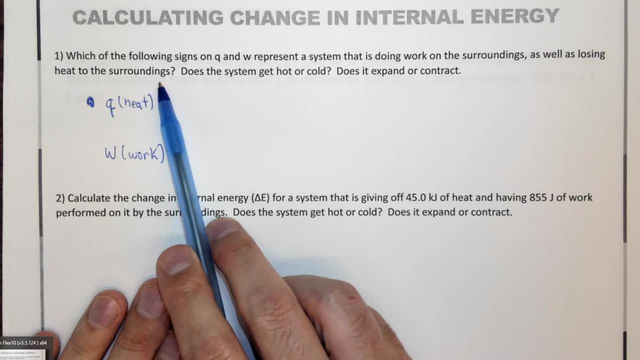 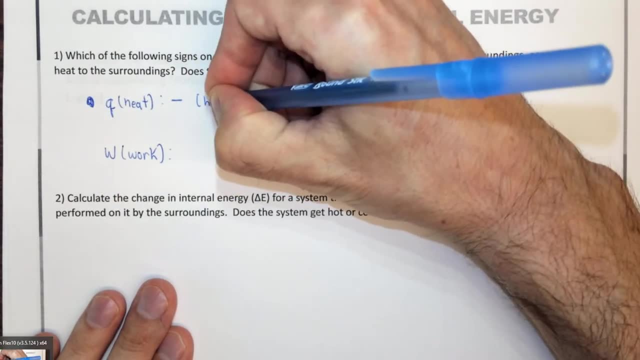 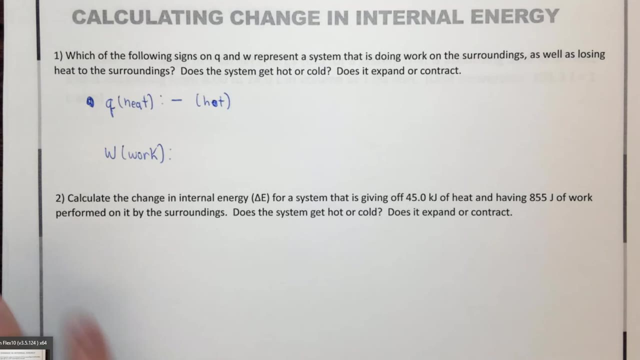 giving off heat. If it loses heat, it's negative And if the Q is negative, this feels hot because if you're losing heat to the surroundings and if you were standing near this reaction, it would feel hot because you are the surroundings and you would feel that heat that it's giving off And the 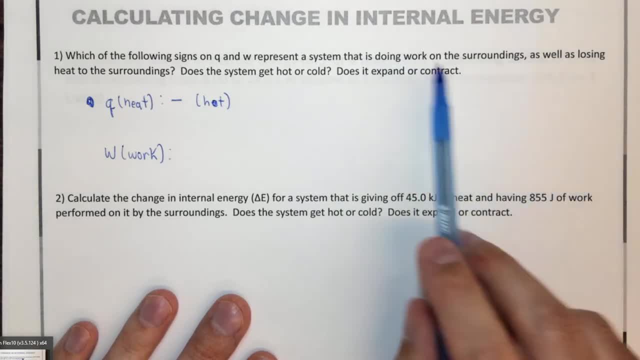 system is doing work on the surroundings. So if it's doing work on the surroundings that means that it is losing work, energy. So W is negative And here we would say for the Q, here the W would feel like if we were starting the. 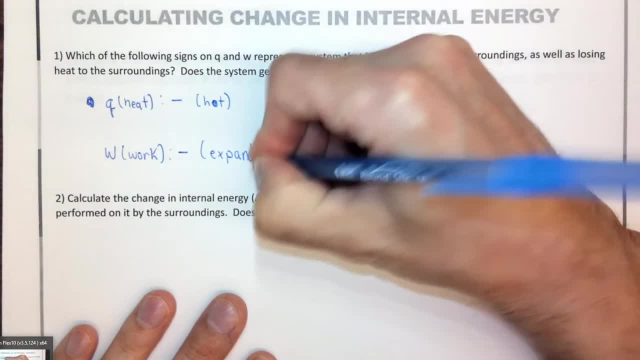 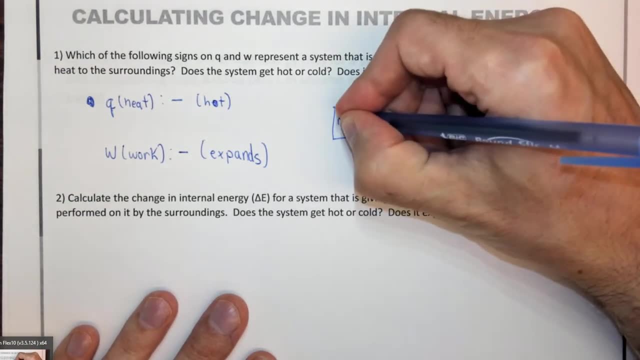 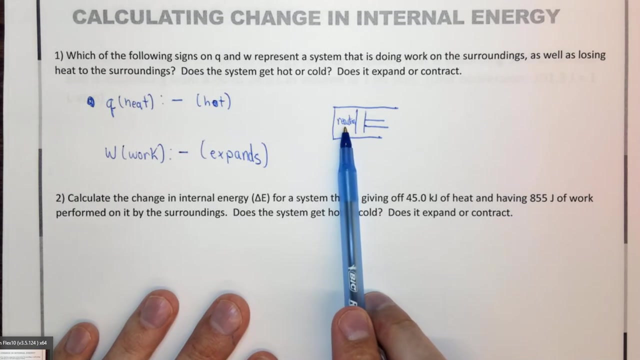 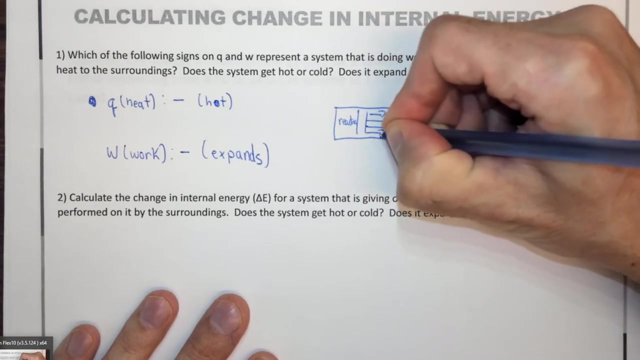 that this expands. So if we thought of this reaction as occurring inside of this piston, right here, what's going to happen? Well, if this reaction is occurring here, which way is the piston going to go? Well, if it's doing work on the surroundings, it's going to push the piston towards the surroundings, Said. 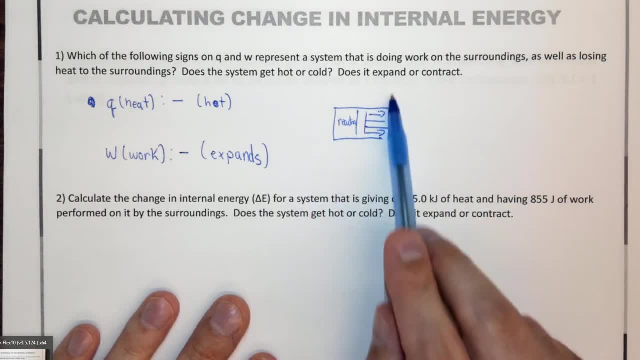 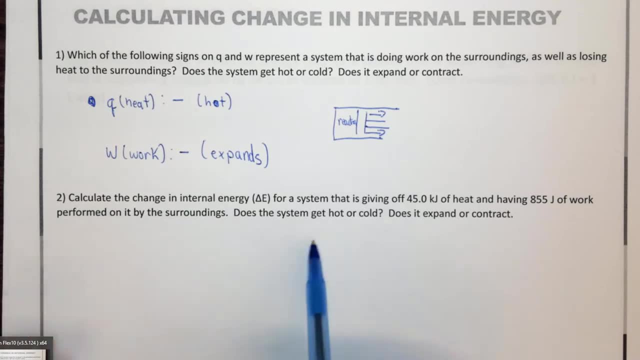 another way. it's going to expand And if you're standing near it it's going to feel hot. So this is basically how heat and work work. The next one is the same thing, except for we actually have numbers. It says: calculate the change in. 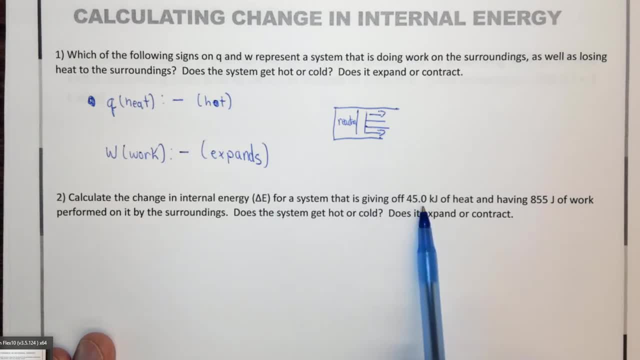 internal energy, delta E for a system that is giving off 45 kilojoules of heat and having 855 joules of work performed on it by the surroundings. So let's look at the equation Again. this is a very simple equation. 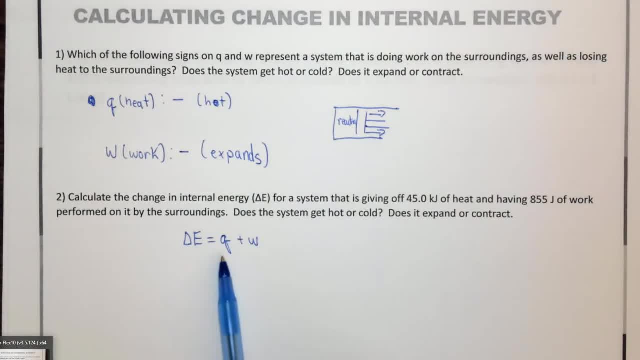 Delta E equals Q plus W. It doesn't get any easier than that, right. We just add two things together. But there's a few tricks. The major trick is determining whether Q is positive or negative and whether W is positive or negative. The 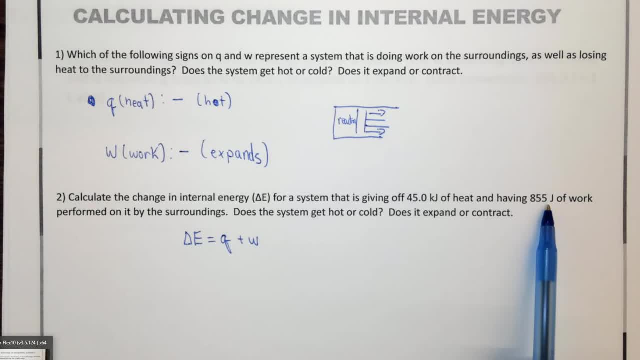 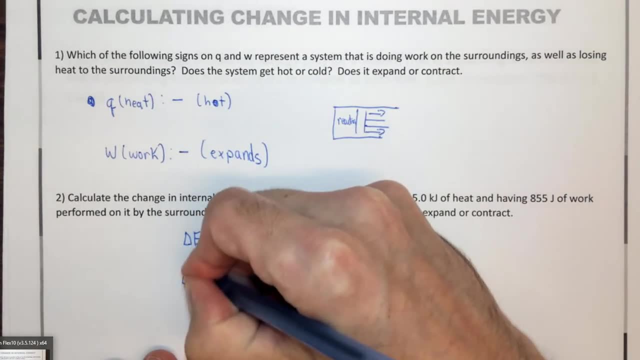 other problem is: this is in kilojoules and this isn't joules, so we need to be making sure we have the same units. So usually delta E's are in kilojoules, so let's use delta E, let's leave the heat in kilojoules, So the system that is. giving off 45 kilojoules of heat on the system is going to speed up. So if we look at the process here, here: so the system that is giving, So the system that is giving off 45 kilojoules of heat on the system, So the system that is giving. 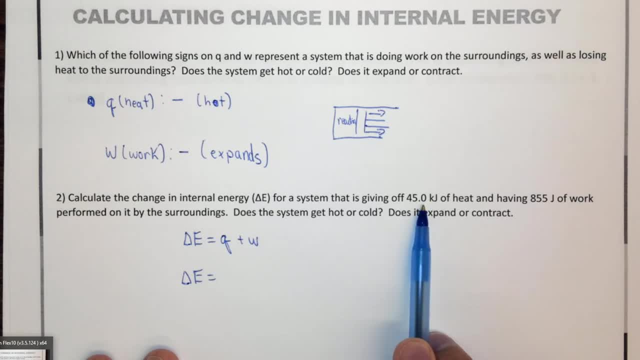 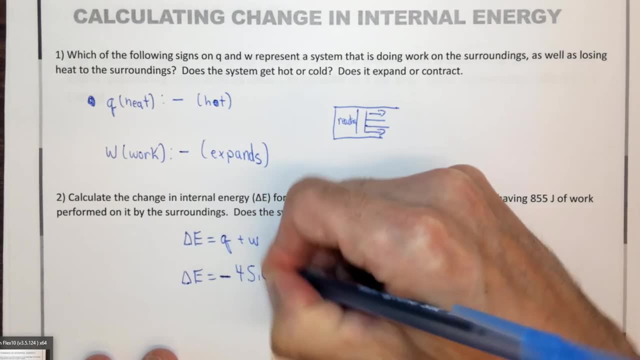 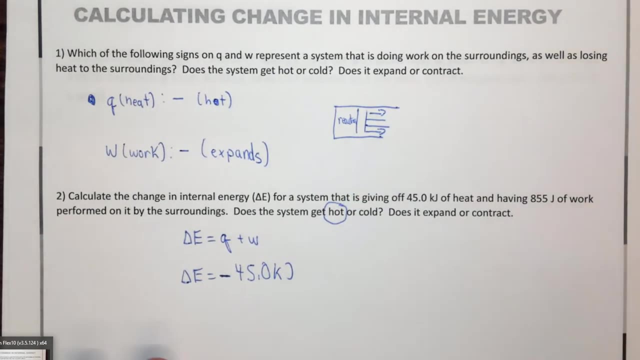 45 kilojoules of heat energy. So it's giving off heat energy, it's losing heat. so if it's losing heat, it's negative 45 kilojoules And this system is gonna feel hot because it's losing heat- to you, the surroundings. you're going to feel that. 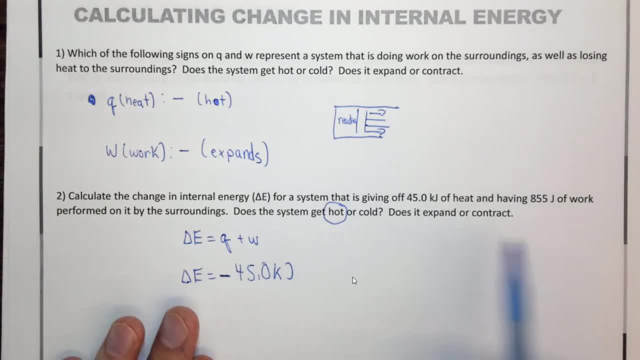 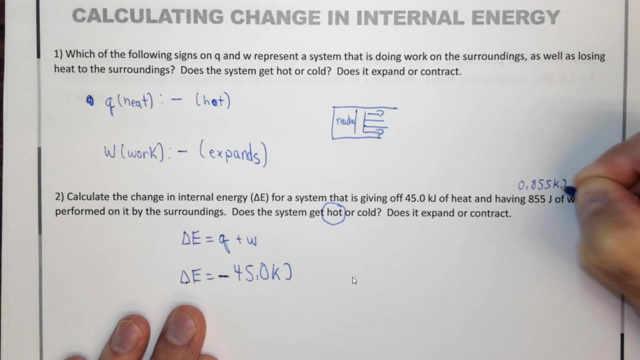 heat, and it's going to feel hot, And it's having 855 joules of work performed on it by the surroundings. Now, first of all, we need to convert this to kilojoules by dividing by a thousand, which is 0.855 kilojoules. Now is it? 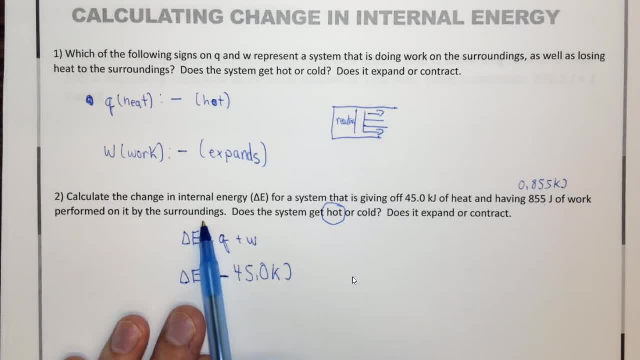 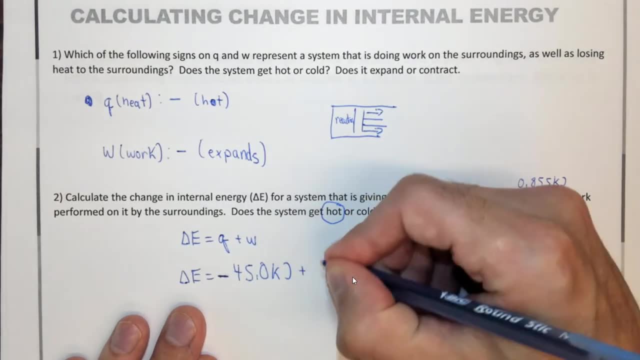 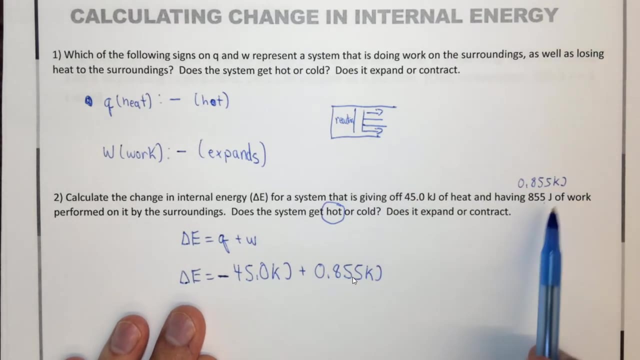 positive or negative. Well, the surroundings are performing work on the system, so therefore the system is gaining work. So if the system is gaining work, it's positive. so we put the 0.855 kilojoules in as a positive number, Since the system is. 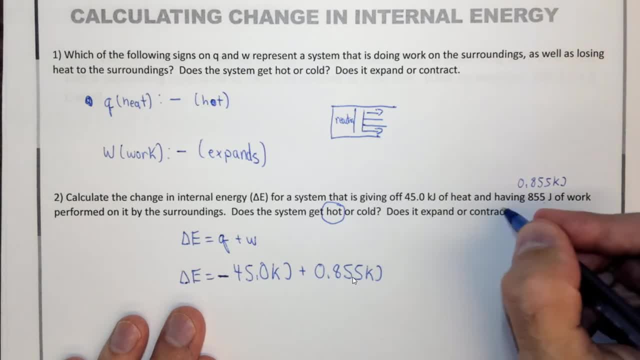 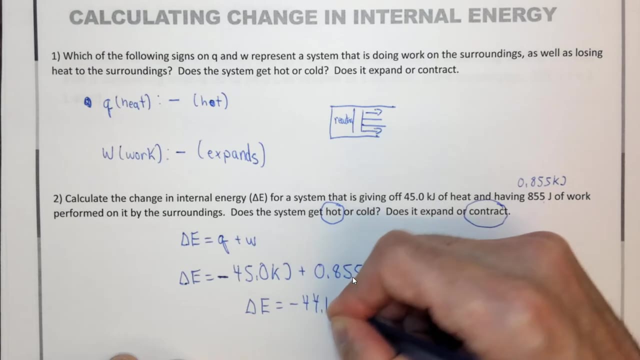 having work done on it and the surroundings are doing the work, it's going to contract. In this case the piston would go in the opposite of the previous case. Now we can add these numbers together. When we add these numbers together, we get that delta E equals negative 44.1 kilojoules. Now it's 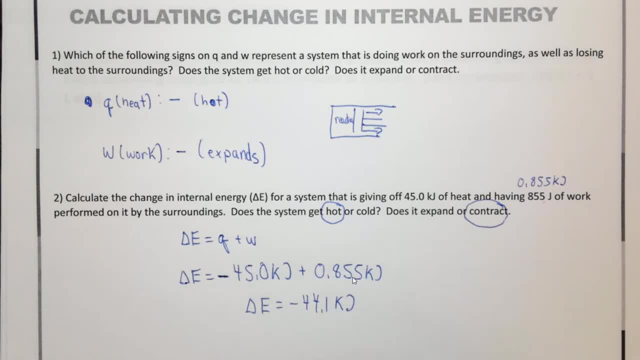 really important to note that that delta E equals negative 44.1 kilojoules. Now it's really important to note that on a multiple-choice test like you would take in this course, all possible answers are going to be there Where this one's positive and this one's. 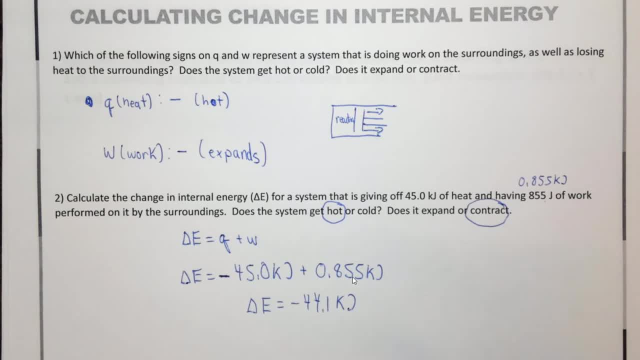 negative, where this one's negative and this one's negative, and so on and so forth. All possible answers will be there. so it's very important to practice with this because, although it seems incredibly simple, it's very important to determine and it's easy to get confused. 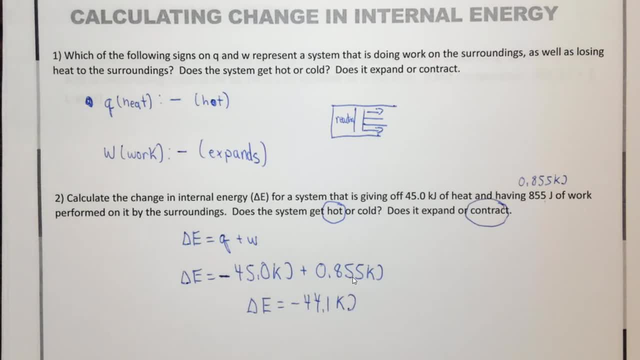 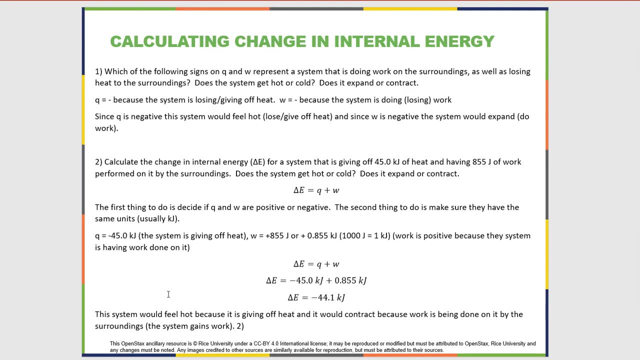 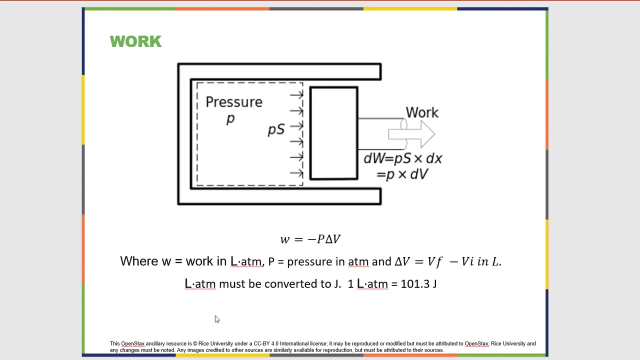 whether they're positive or negative. The best way, like anything, is to practice several of them Alright. so now that we've looked at calculating the change in internal energy, let's talk about the two variables, heat and work, basically separately. So the first one we want to talk about is work. So work is basically. 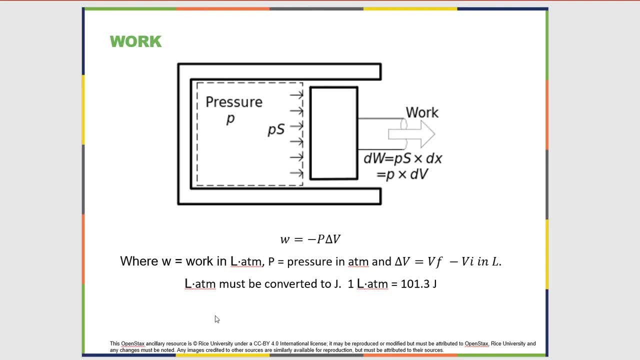 the energy of motion, alright, so some physical motion has to occur. Chemical reactions don't always do work. When they do, usually a lot of gas is generated, so they expand. If you have a reaction, that's, you know, a solid and a 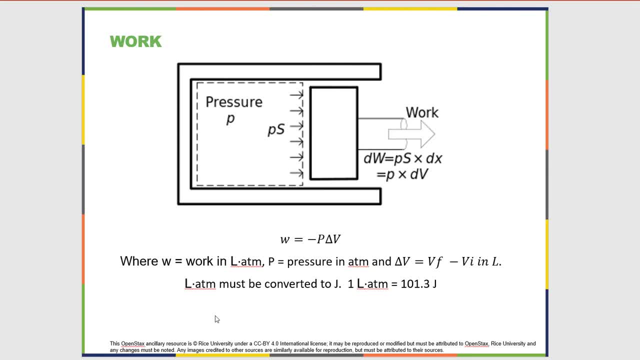 liquid and it generates a gas, or two liquids that generate a gas or whatever. if a gas is generated, the system will expand and that will do work For reactions which have a lot of work done on them. generally speaking, gas is consumed, So if a bunch of gas is consumed, so 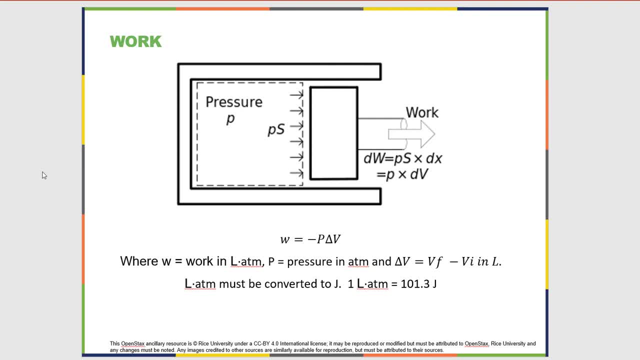 there's less gas, then the piston will move in and work will be done on it. So in this case, where the piston is moving out in this direction, okay, the system is doing work and it's losing work, so work is negative. In the opposite case, where 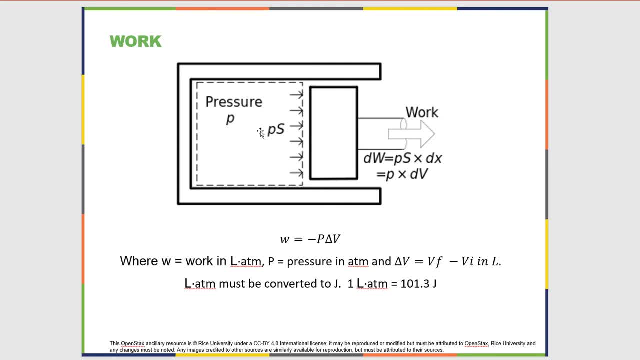 the piston is moving in, the system is having work done on it, the surroundings are pushing against the system and work is positive for the system. And we can use this formula for pressure-volume: work Work equals negative P. the pressure in atmospheres. delta V, where this is the change in volume: VF minus VI in. 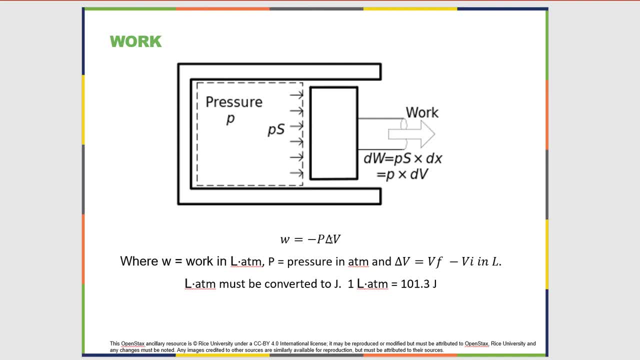 liters. Notice that you're gonna have pressure in atmospheres times volume in liters, so you're gonna get liter atmospheres as your unit. A joule, excuse me, one liter atmosphere is 101.3 joules, So you may need this conversion in order. 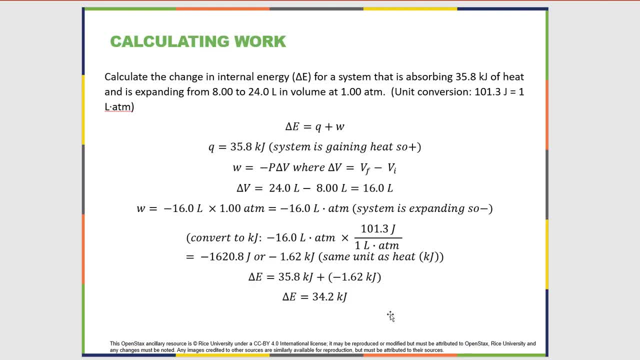 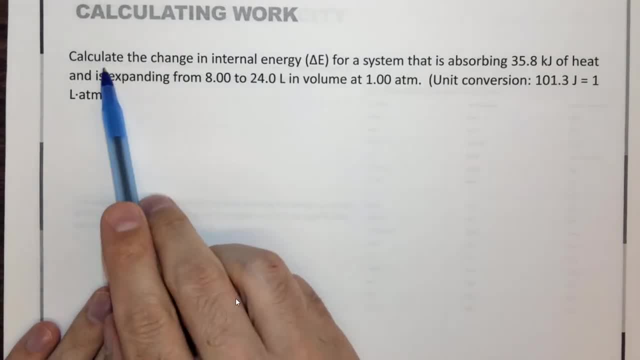 to convert the work to joules. So let's look at an example, and again I'm going to switch over to the writing part. So it says: calculate the change in internal energy delta E for a system that is absorbing 35.8 kilojoules of heat and is expanding from 8 to 24. 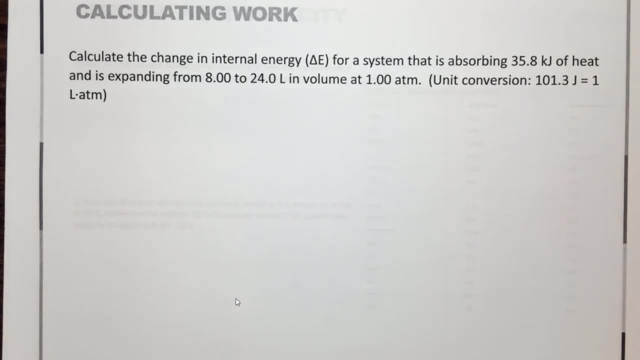 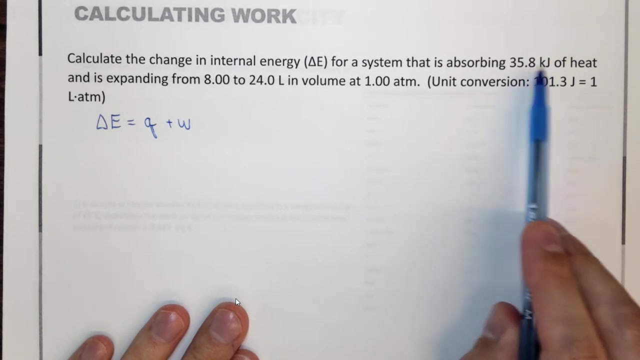 liters in volume at one atmosphere of pressure. So, as you know, delta E equals Q plus W. Well, let's look at Q. In this case, the system is absorbing 35.8 kilojoules of heat energy. So 35.8 kilojoules is being absorbed. That means 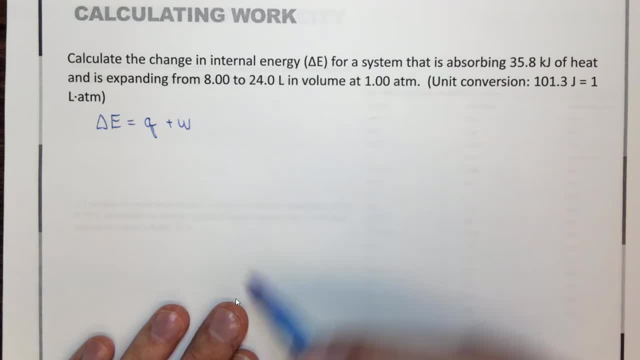 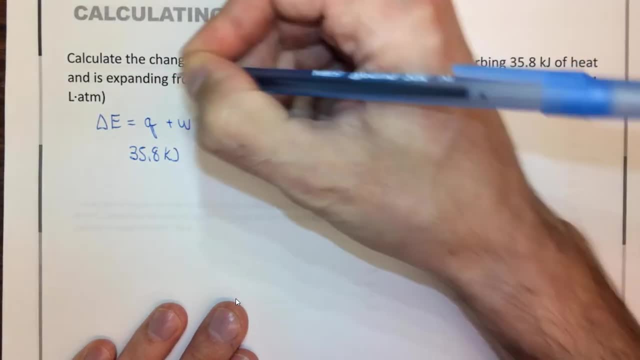 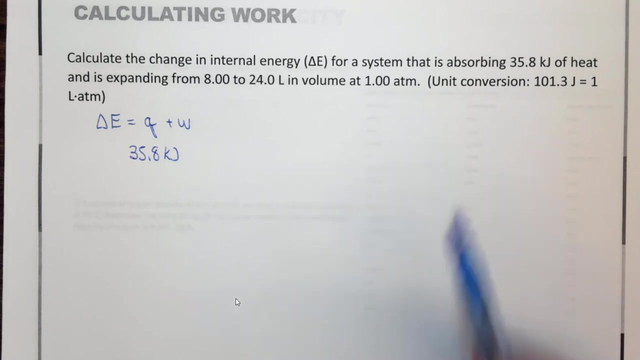 the surroundings are giving heat energy to the system, So the heat energy is positive. So this is 35.8 kilojoules of heat energy as a positive number. If you were standing near this, it would feel cold. Next we want to look at W, and W equals negative. 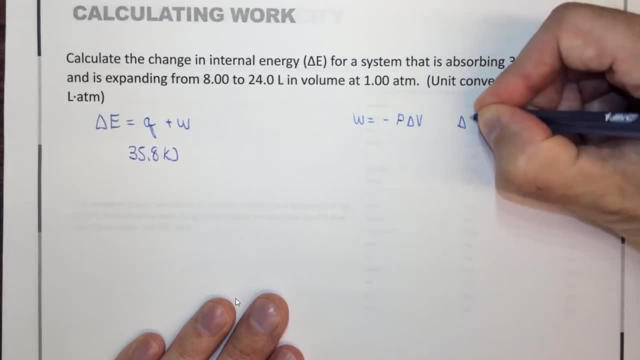 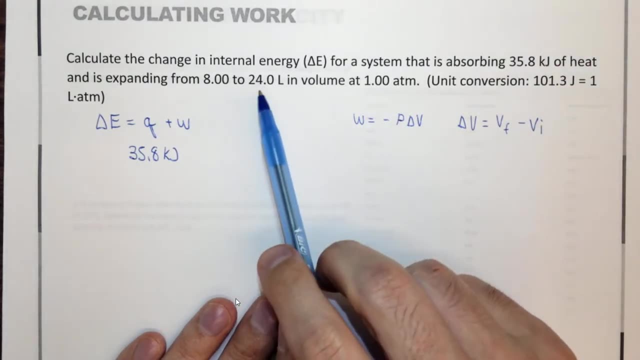 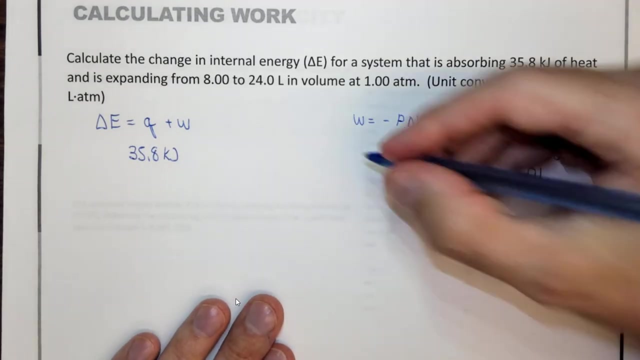 W equals negative, W equals negative W. Penglong V, where delta V equals VF minus VI. So in this case we have the final volume, 24.0 liters, minus the initial volume, 8.00 liters, which is 16.0 liters, as the change in volume and the pressure is one atmosphere. So work equals negative P one. 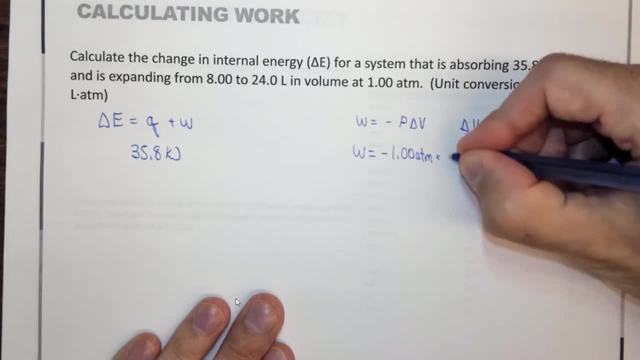 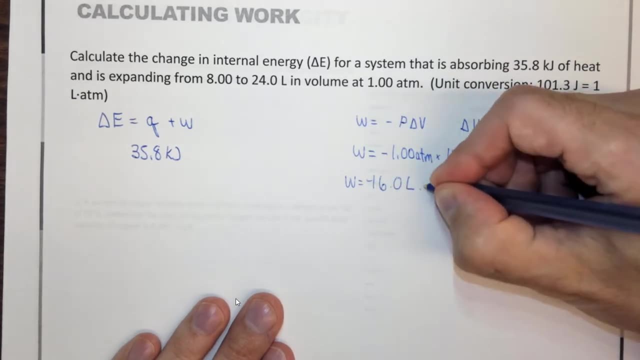 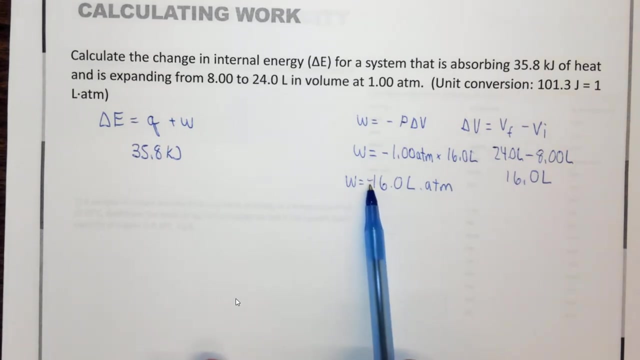 atmosphere. delta V: 16 liters work equals 16, negative 16, liter atmospheres. Notice: does it make sense that the work term is negative? Always, always, double check yourself, Just like in the previous examples, whether these are negative or. 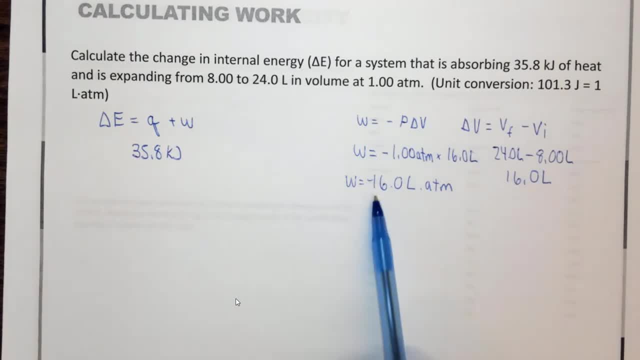 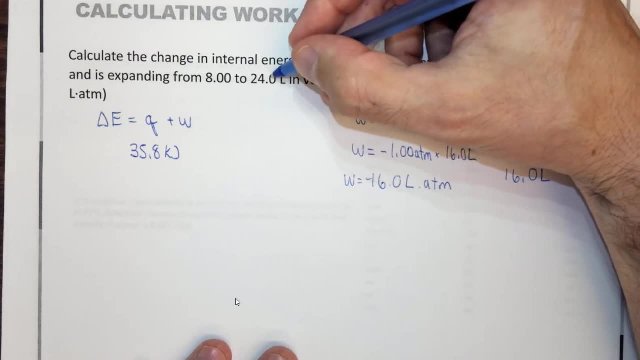 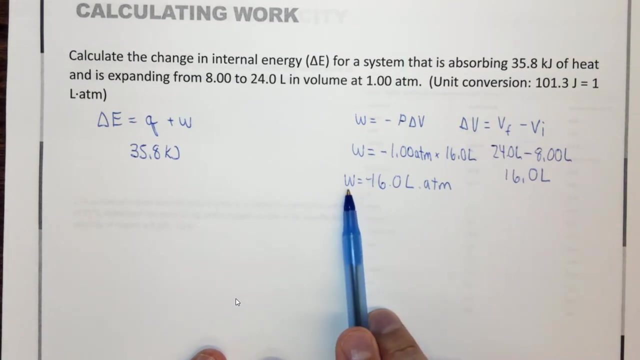 positive completely influences the answer. So does it make sense that this is negative? Well, yeah, it does, Because it started off at 8 liters and expanded to 24 liters, So the system did work on the surroundings. If the system does work, the system loses work. so the 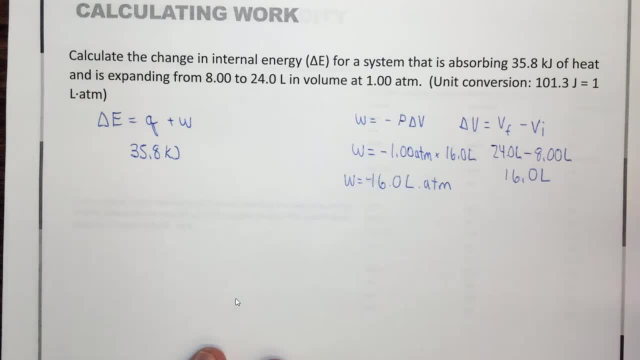 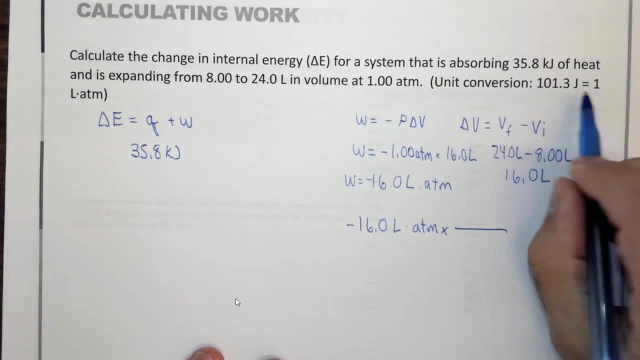 work term has to be negative. Now we need to convert this liter atmospheres to kilojoules. So we take negative 16.0 liter atmospheres times, there's 101.3 joules in one liter atmosphere. so we put the one liter atmosphere on the bottom. 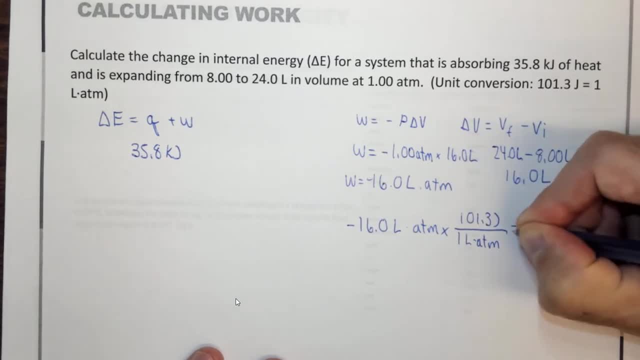 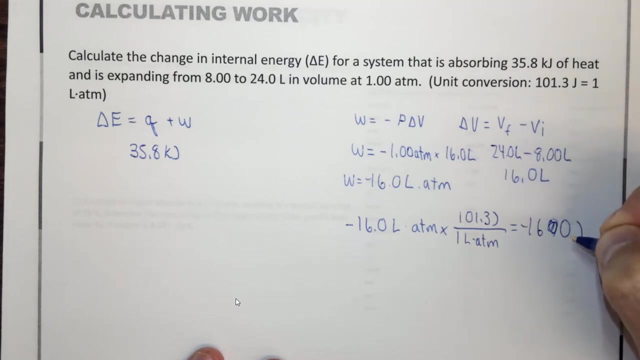 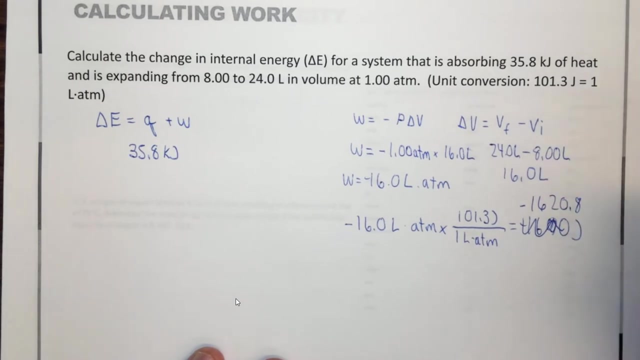 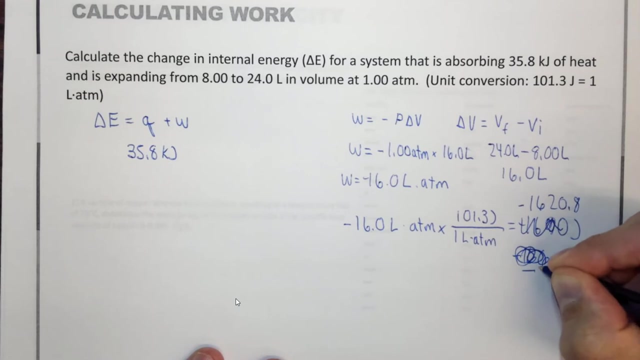 the 101.3 Joules On the top and we find that this is one negative one six zero zero joules, And I should be careful here. sorry, this is negative one six, two zero point eight And if we round it to three sig figs it'd be negative one sixty two. negative one six. 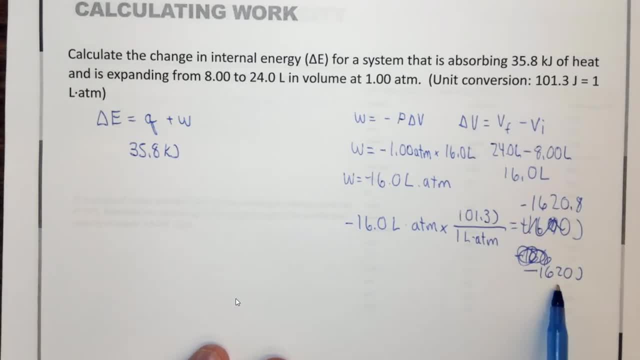 two, zero joules. We need to convert that to kilojoules by divided by a thousand. so we plug in negative one point six, two kilojoules. Now we take the thirty five point eight, we subtract the one point six, two and we find that delta E the. 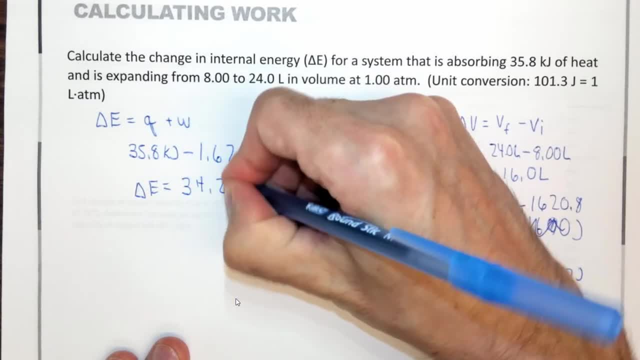 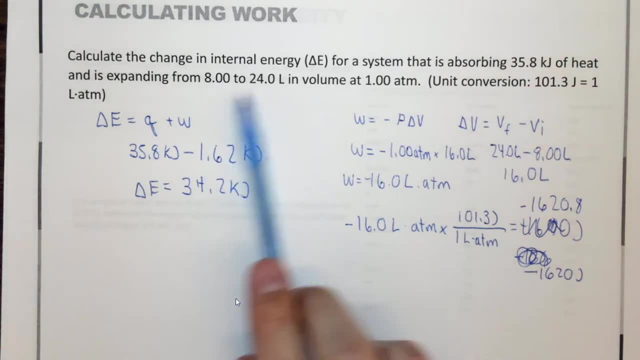 change in internal energy equals thirty four point two kilojoules. So this is how we could calculate internal energy if we're given pressure-volume work. This is called pressure-volume work because we're given a pressure and a change in volume, So this is the work term. The next thing, of course, we want to look at, 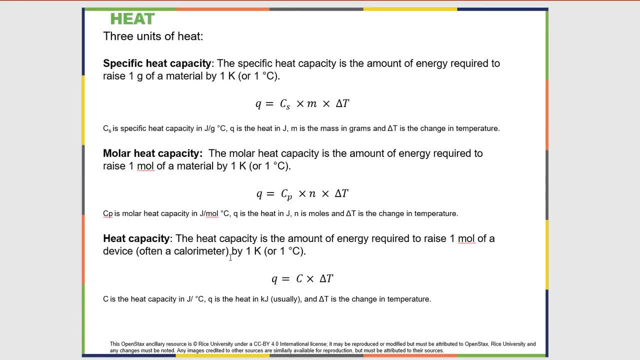 is the heat term. Unfortunately, for the heat term, there are several things going on here for the heat term. So Q is heat and there are three major units of heat. There is one using the specific heat capacity, one using the molar heat. 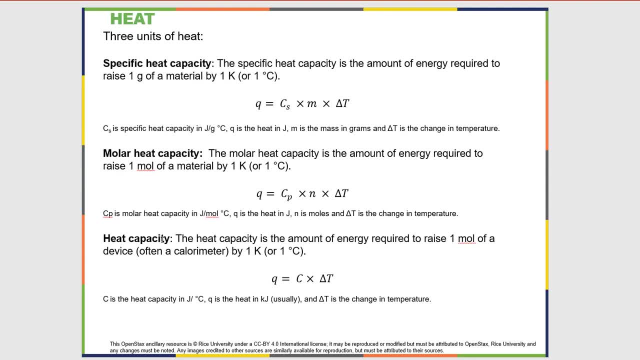 capacity and one using the heat capacity, And these things are all a little bit different and they're used for different applications. So the specific heat capacity is the amount of energy required to raise one gram of the material by 1 K or 1 degree C. Note that a change in temperature. it doesn't. 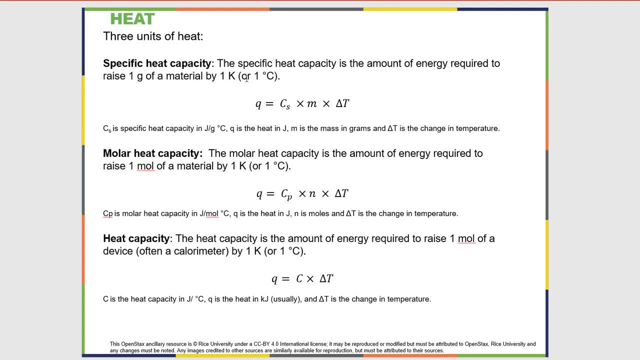 matter if it's C or K, because the units are the same. So a change from 273 to 274 is 1 K, a change from 0 to 1 degree C is 1 degree C. The change in temperature is the same, they're both 1, 273 is 0 Celsius, 274 is 1 Celsius. So 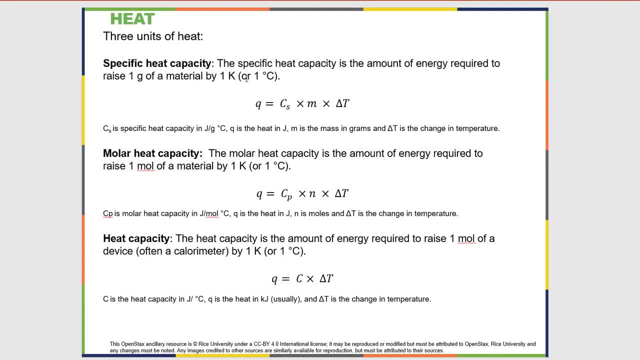 they're basically the same thing, so you don't have to worry about that. So the specific heat capacity is commonly used and the reason that it's important is because it takes into account the amount. So the specific heat capacity is in joules per gram degree C. 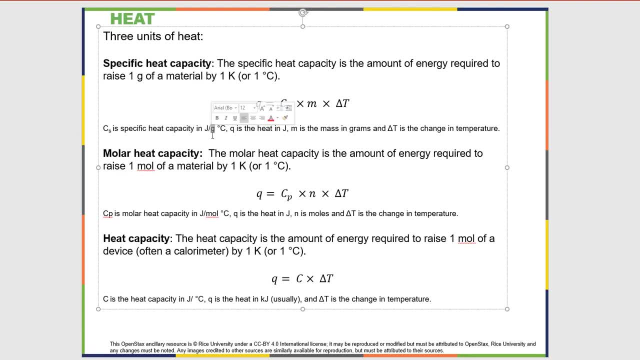 So for every gram of the substance a certain amount of joules will cause a certain temperature change, And this is an empirically measured thing for different substances. and it turns out that water has an extremely high specific heat capacity, so it takes a lot of energy to raise the temperature of 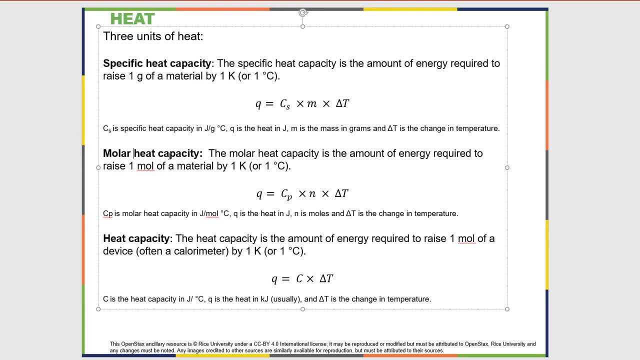 water. The molar heat capacity is almost the same as the specific heat capacity. the only difference is: instead of grams as the amount term, moles are the amount term, So you could imagine that chemists use this because they want to know it in terms of moles for the amount term instead of grams, as. 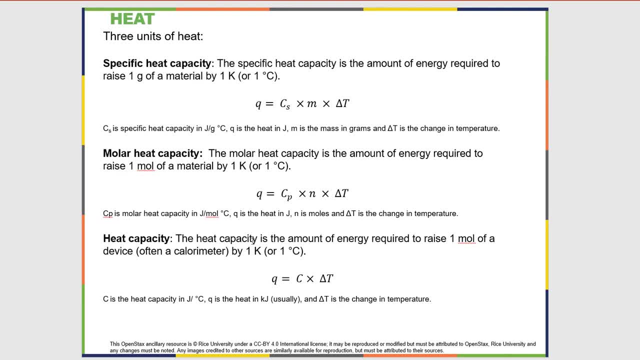 the amount term. The heat capacity is interesting and we'll talk about it a lot more in the next section. in fact, we won't do any specific examples of the heat capacity in this section because it usually works with a bomb calorimeter. This does not have an amount term, this is just C, delta T, and this is 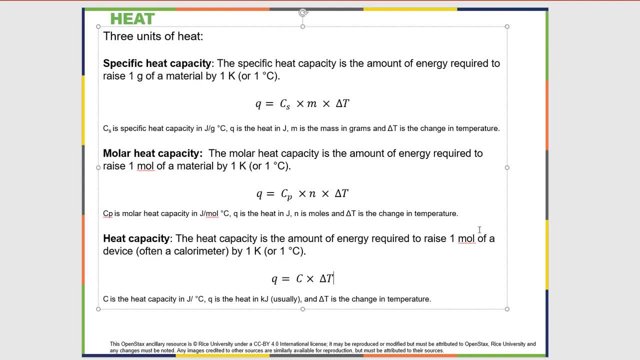 usually used. this shouldn't be one mole, this should be just to raise the temperature, raise the temperature of a device, often a calorimeter, by one K. So let me try this again. So Q here equals the C times delta, T, Here there's no. 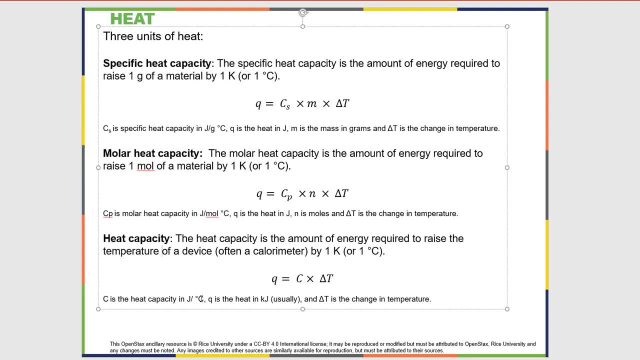 amount term, it's just joules per temperature change. This is used for devices like bomb calorimeters, where it's made up lots of different materials, so you wouldn't want to use molar heat capacity or specific heat capacity, because these are specific to different materials like 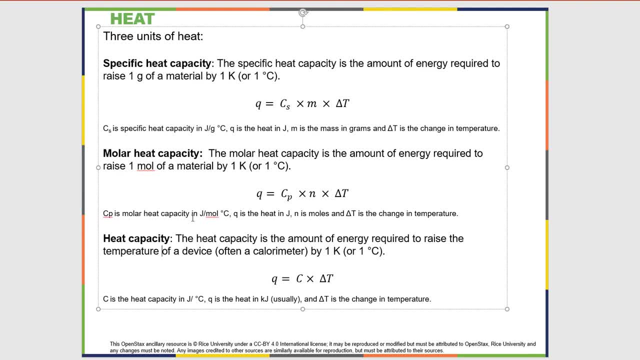 water or aluminum or whatever the case may be. so that's basically why you would use this if it's made out of many different materials. This is used if, for example, one were to want to know how much how many calories are in a French. 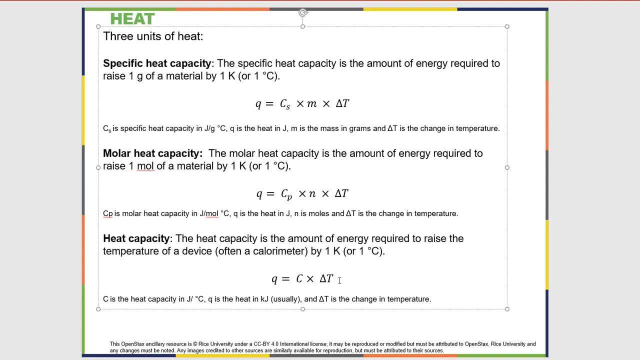 pie. All right, you could burn a french fry in the presence of pure oxygen. figure out how much calorimeter heats up and, based on how much the calorimeter heats up, you can determine the amount of calories that were in the original french fry. And 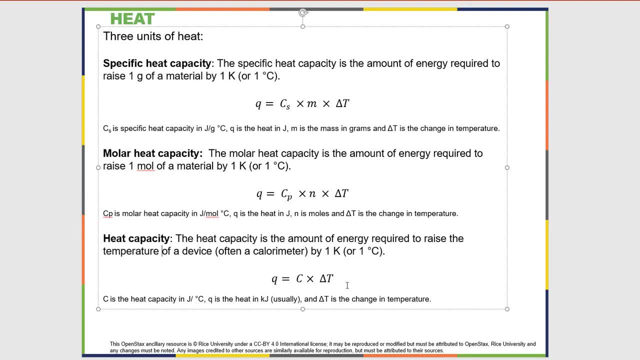 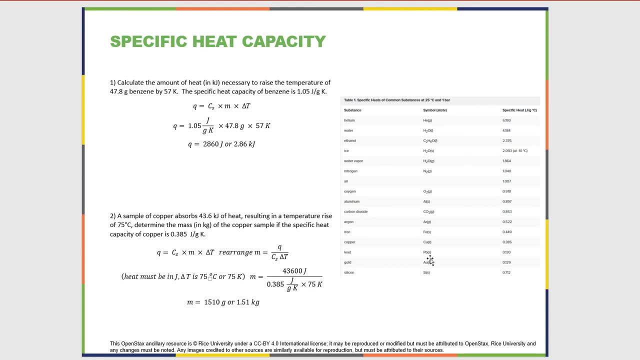 we'll talk about this one a lot more in a few minutes in the next section. So let's look at the specific heat capacity. So if we look here, these are the specific heat capacities of some different substances. So aluminum is 0.897 joules per gram degree C. Water is 4.184 joules per gram degree C. 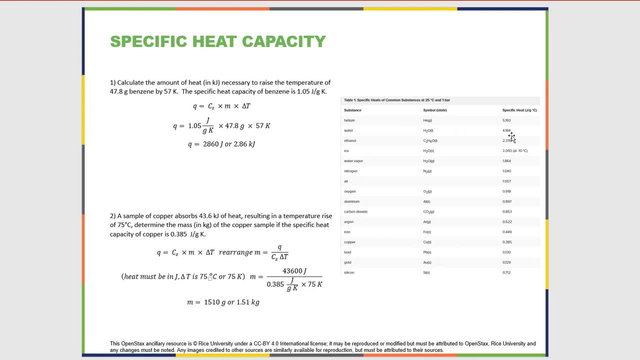 So there's a couple of things to take into consideration when we're looking at these specific heat capacities, and then we'll do a couple of mathematical examples. First of all, the amount matters, right? So if you want to heat up a little, 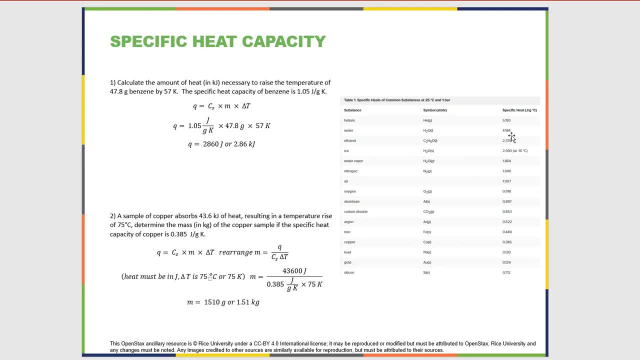 bit of water, you add a little bit of energy. If you want to heat up a lot of water, you have to add a lot more energy. So if you want to heat up a lot of water, you have to add a lot more energy. 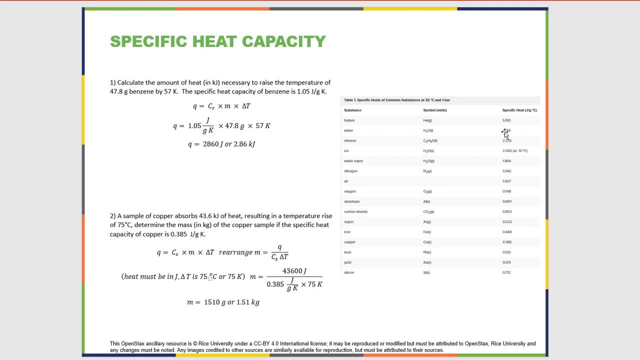 So if you want to heat up a lot of water, you have to add a lot more energy. So there is a gram term. so the more water you want to heat up, the more energy it requires. The second thing is that different substances have different 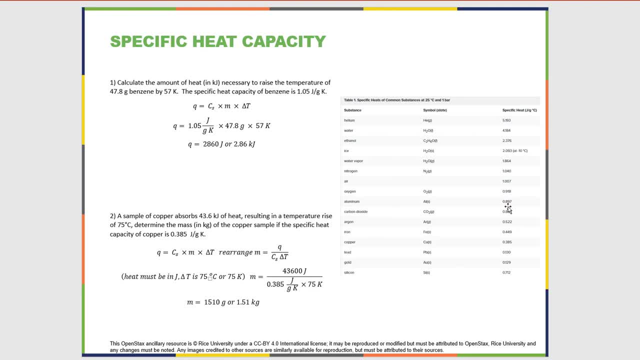 specific heat capacities. So in order to change the temperature of aluminum by 1 degree C, for each gram you have to add 0.897 joules. For each gram of water you have to add 4.184 joules. So if you think about this, if you take a pan, say: 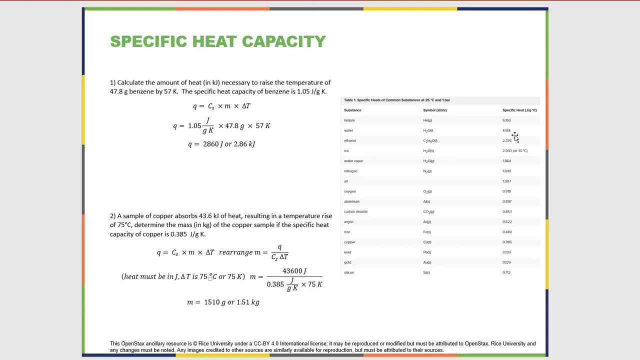 it has a mass of 1 kilogram and you put it on a burner on the stove. if you leave it for two minutes, if you add two minutes worth of heat to it, its temperature will change enough that you can no longer touch it. If you take that same pan and you add a liter of water to, 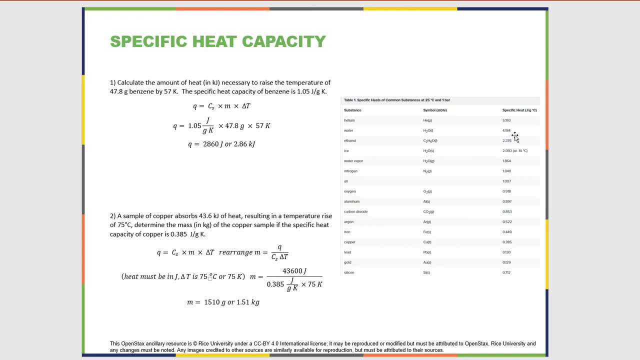 it and then you heat it for two minutes. you could probably still touch the pan, because the temperature of the water will not change nearly as much as the temperature of the pan, And the reason for that is the specific heat capacity of water is much higher. 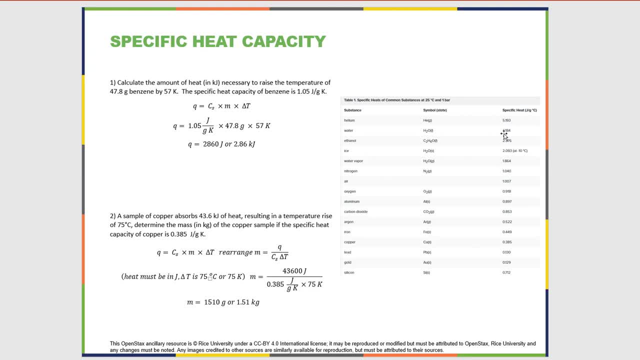 So two things to take into account: one, that the amount matters: the more water you heat up, the more, the more energy it requires. that's obvious. And the second one is that different substances have different specific heat capacities and therefore their temperature changes will be different, even if the same. 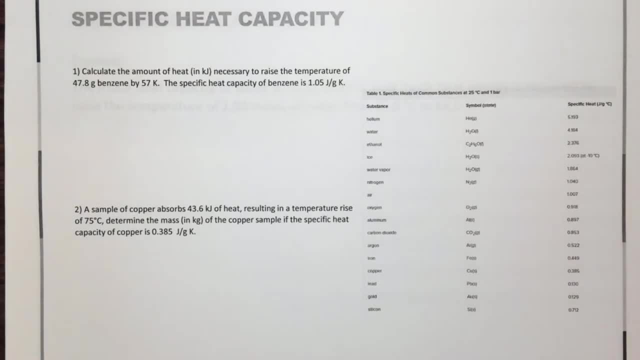 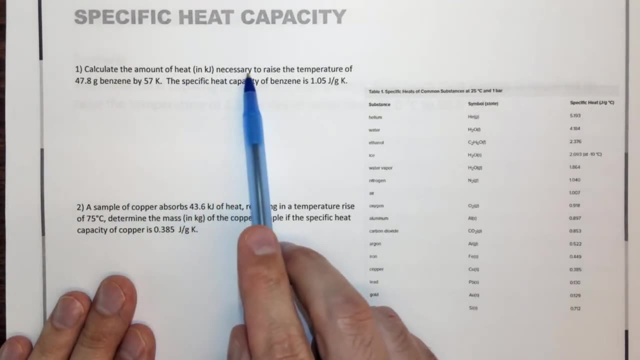 amount of energy is applied. So let's look at a couple of examples here of things we can calculate using these specific heat capacities. So it says: calculate to raise the temperature of 47.8 grams of benzene by 57 K, The specific heat. 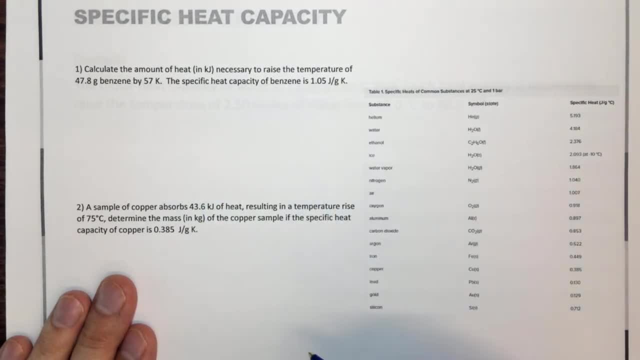 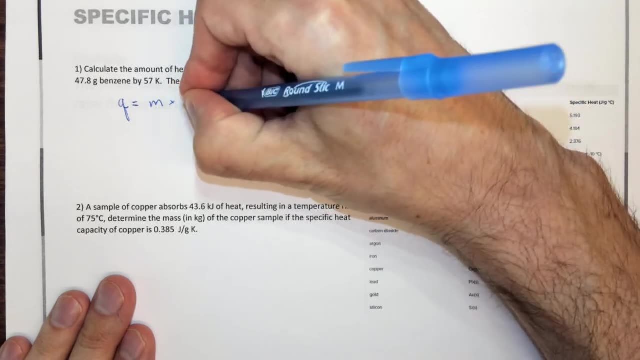 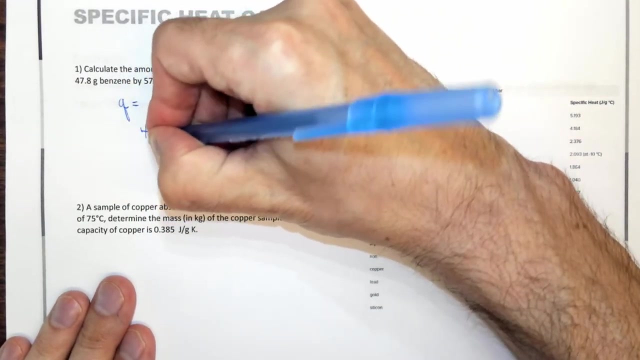 capacity of benzene is 1.05 joules per gram K. So here Q equals mass, which has to be in grams times specific heat capacity times change in temperature. So we can plug in the mass in grams: 47.8 grams times the specific heat. 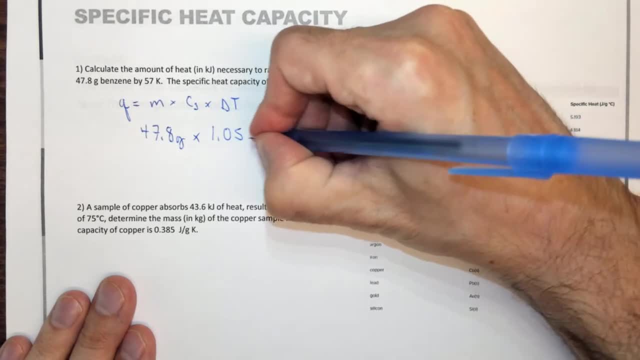 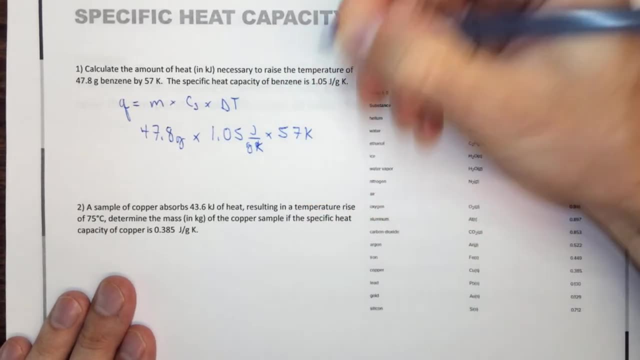 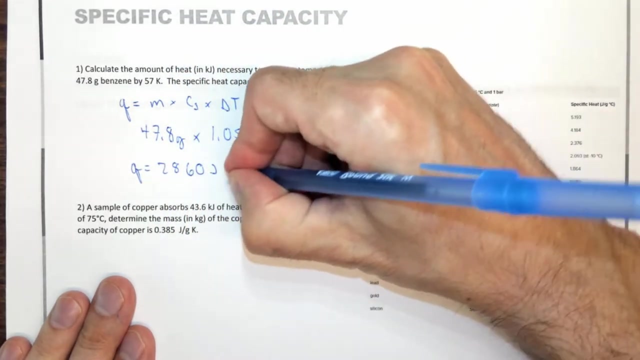 capacity of benzene, which is 1.05 joules per gram degree C or K times the temperature change, 57 K. When you do this you find that Q equals 2860 joules, or if you want to convert that to kilojoules because it asks for it in: 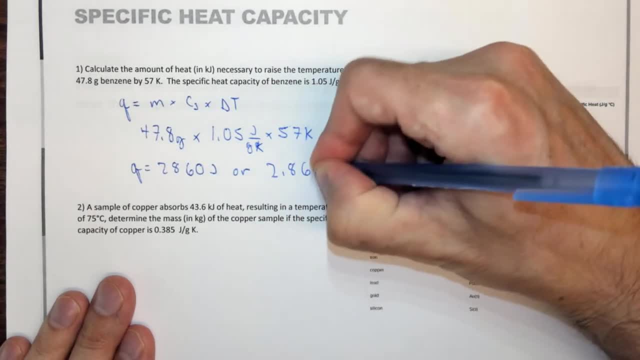 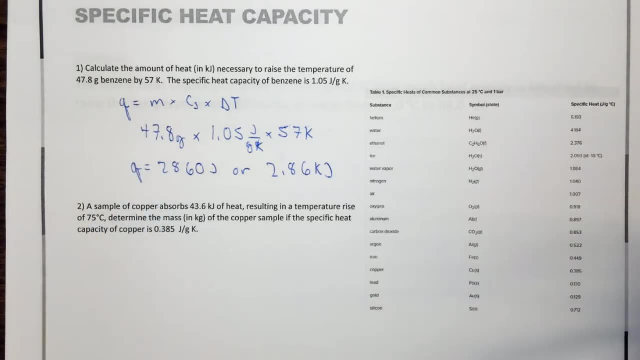 kilojoules divide by a thousand 2.86 kilojoules. So this is an example of finding Q. Remember, in the previous example we found delta E and W. Now one thing to note is this: Q positive or negative? Well, we're heating up benzene. If you're heating something, 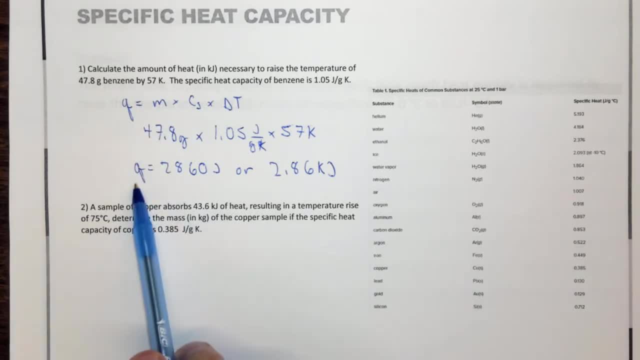 up. you're putting energy in, so Q with respect to the benzene must be positive. Next question: it says a sample of copper absorbs 43.6 kilojoules of heat, resulting in a temperature rise of 75 degrees C. Determine the mass in kilograms of the copper sample, if the 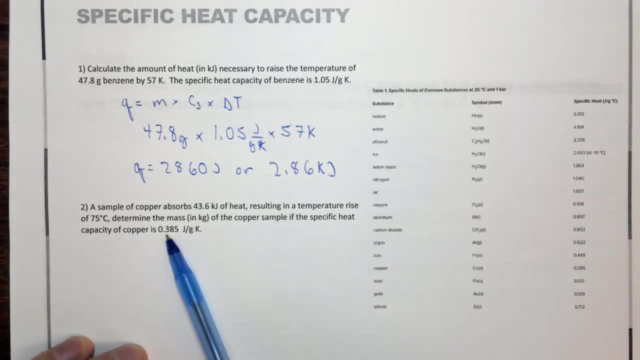 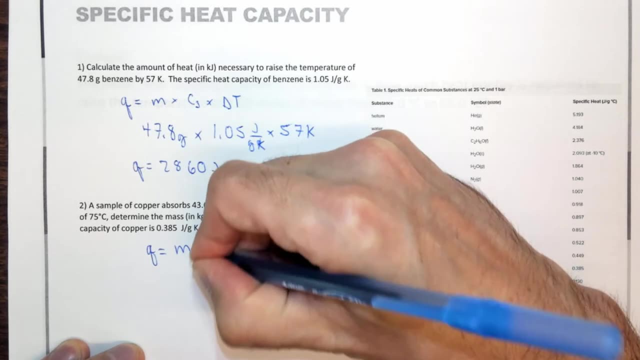 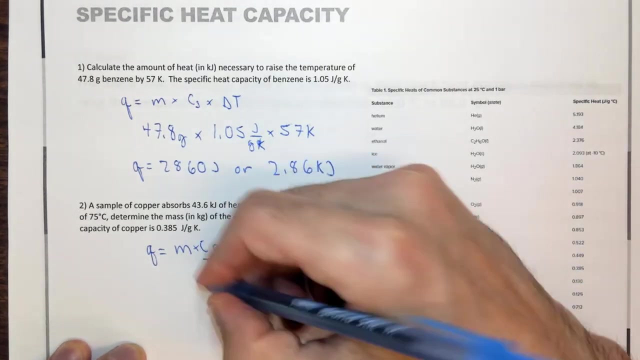 specific heat capacity of copper is zero point three eight five joules per gram K. So Q equals mass times, specific heat capacity, times, change in temperature. Notice: here we're trying to find M, so we need to divide by C, sub S, delta, T And we 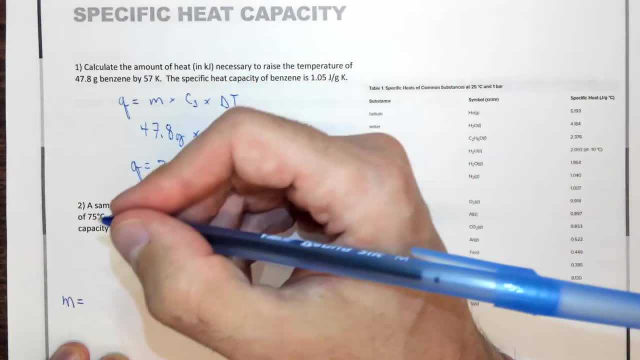 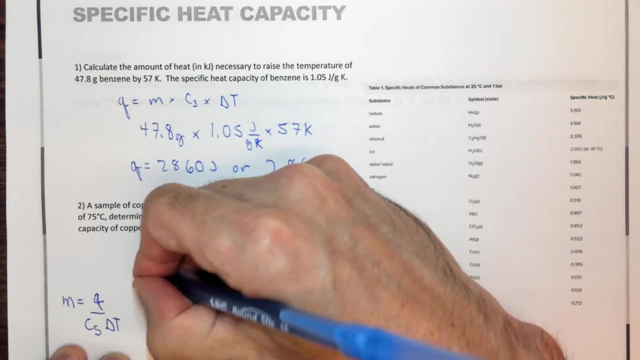 can rearrange this equation as mass equals C sine W times the heat capacity of copper Q divided by C sub s delta T. So we just divided both sides of the equation by C sub s delta T And we got this new equation just rearranged. So now we need 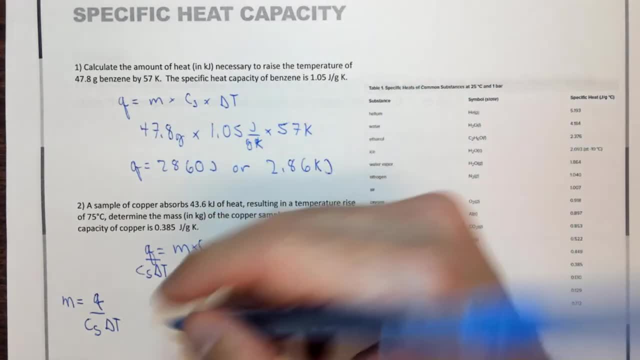 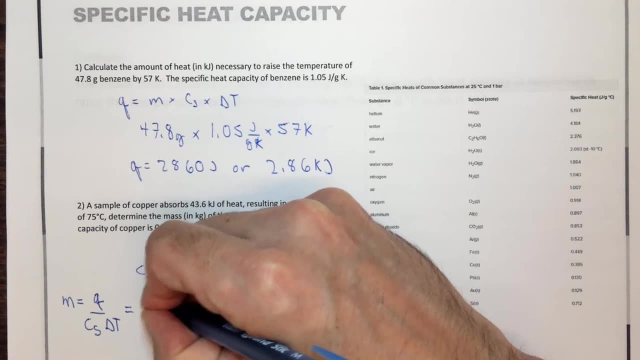 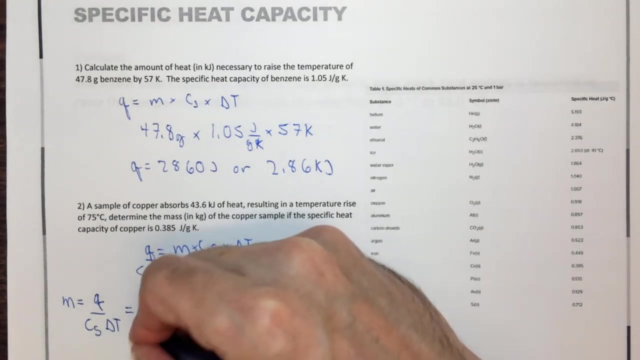 to find the answer here. Remember that Q has to be in joules, so don't plug in the 43.6 kilojoules. Put in 43,600 joules divided by the specific heat capacity: 0.385 joules per gram k or degree C change in temperatures doesn't. 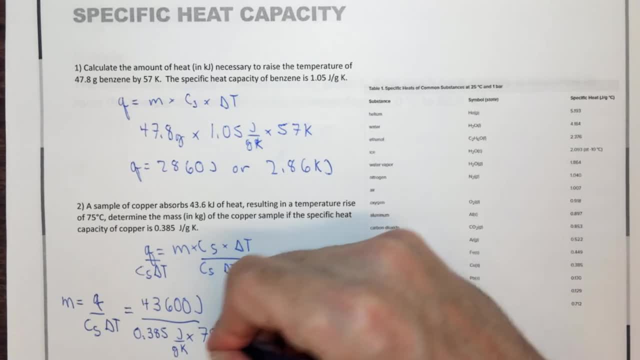 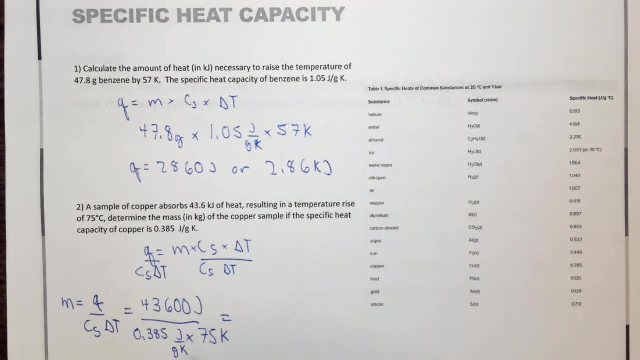 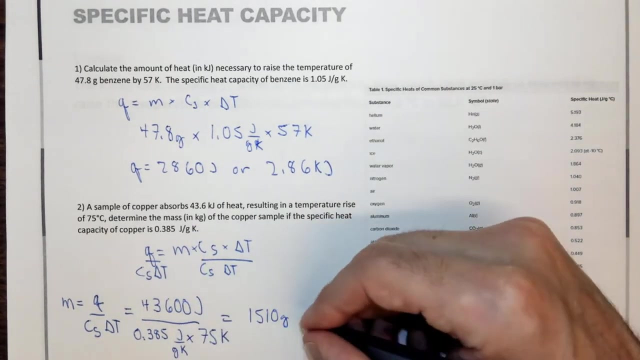 matter times. the change in temperature, which is 75 degrees C or 75 k. Again, it's a change in temperature, so it doesn't matter which unit it is in. When you do this math, you find that the mass is 1510 grams, or it asks for it in kilograms. 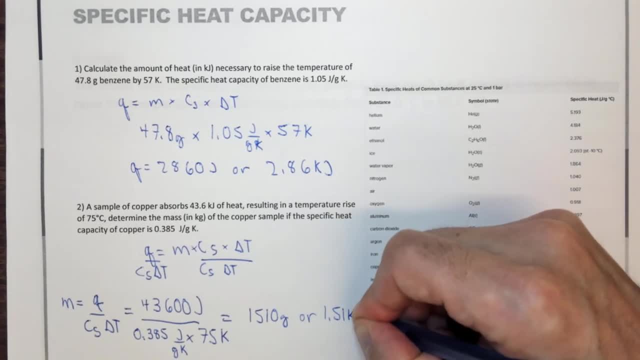 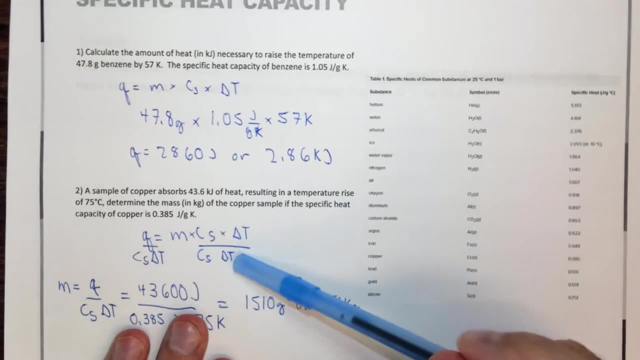 divided by a thousand, which is 1.51 kilograms of copper. Now I'm going to show you how to do this. So what I'm going to do is I'm going to. So these are ways we can either calculate Q or we can use Q to calculate. 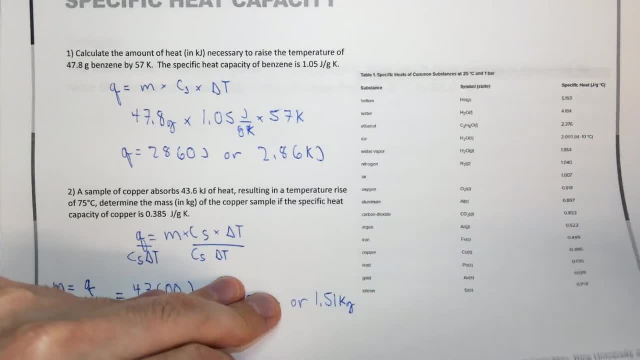 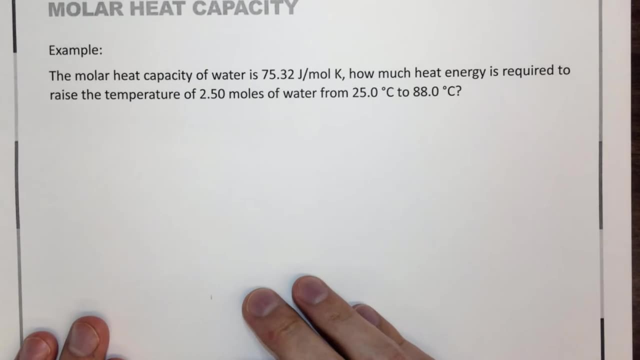 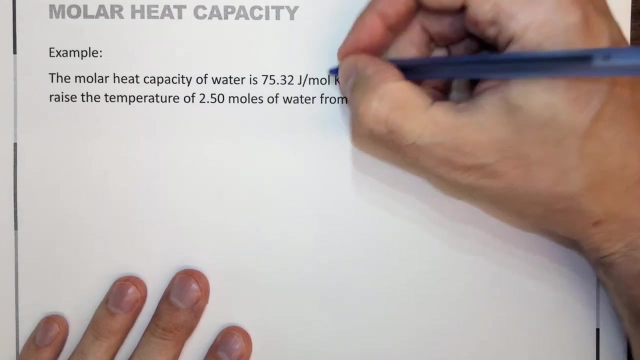 the mass of an object. Now, in the next section we want to look at the molar heat capacity, and the molar heat capacity is the same as the specific heat capacity, with one key difference: It's joules per mole K. so if this was, 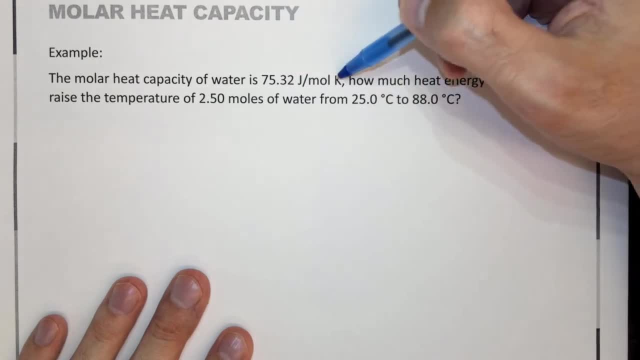 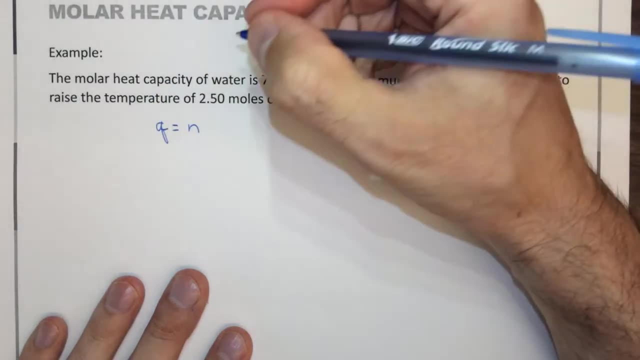 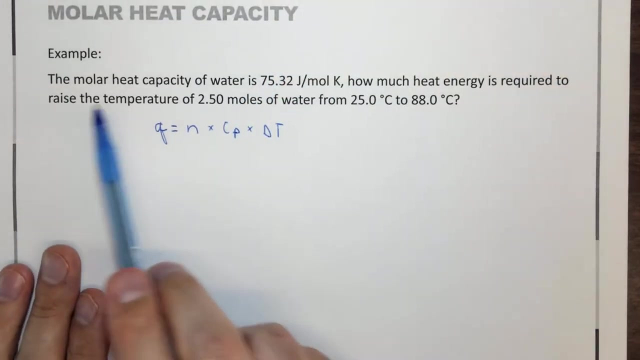 specific heat capacity. this would be grams, but because it's not, it's moles. So in this case Q equals N, which is moles times Cp, which is the molar heat capacity times delta T. So let's read the question: The molar heat capacity of 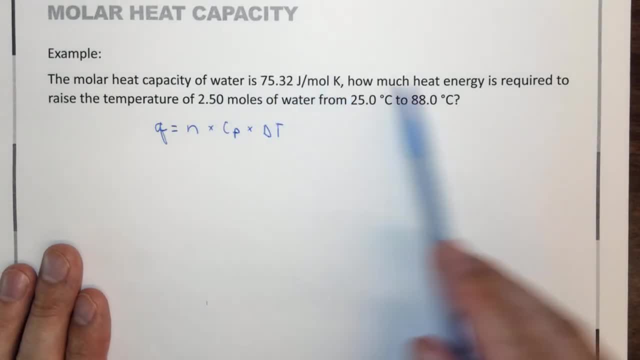 water is 75.32 joules per mole K. How much heat energy is required to raise the temperature of 2.5 moles of water from 25 degrees C to 88 degrees Celsius? Alright, so this is basically what we have. 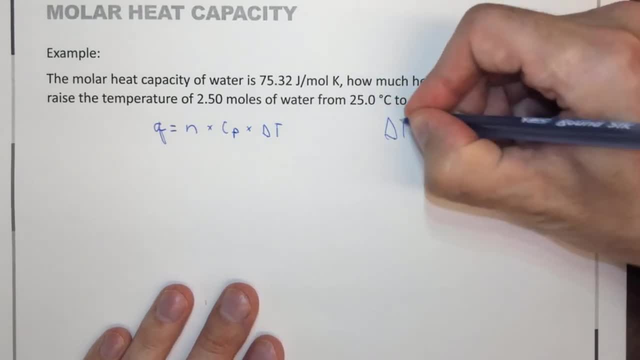 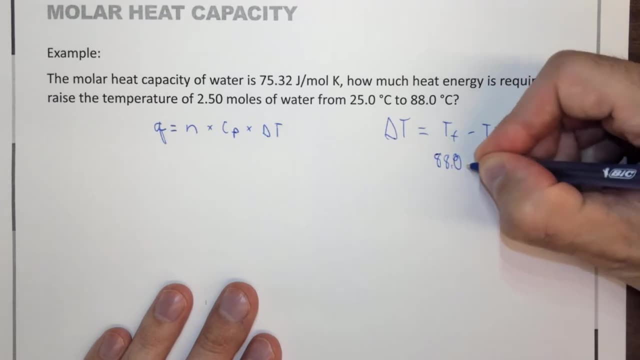 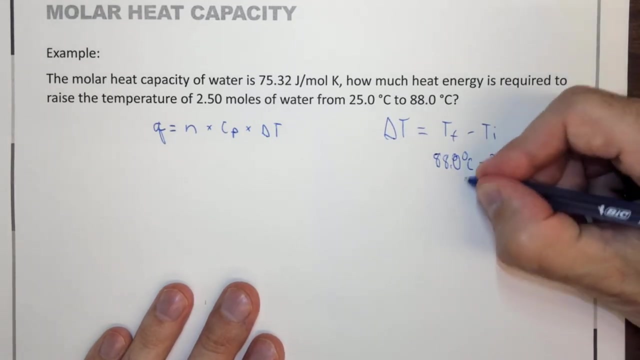 to do. Well, in this case we're not given the change in temperature, so we have to find that delta T equals Tf minus Ti. so we take the 88 degrees, 88.0 degrees C minus the 25 degrees C, and we do that subtraction. we find that it's 63.0. 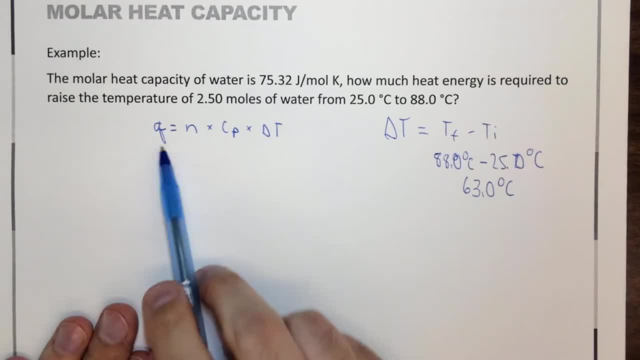 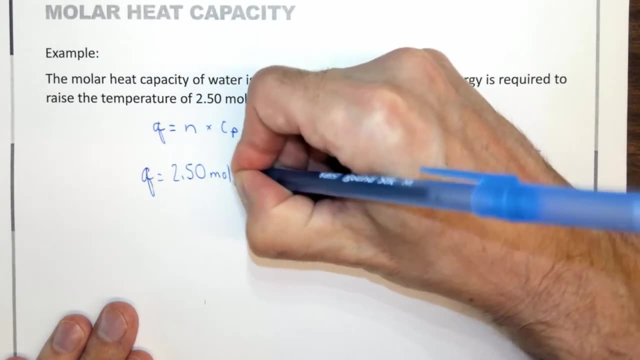 degrees C is the change in temperature. Now we can plug in: Q equals N, the moles, 2.50 moles times N. Now we have to know, in this case, the molar heat capacity: 75.32 joules per mole K.